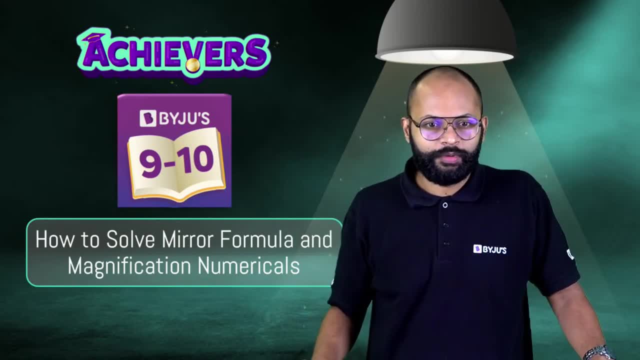 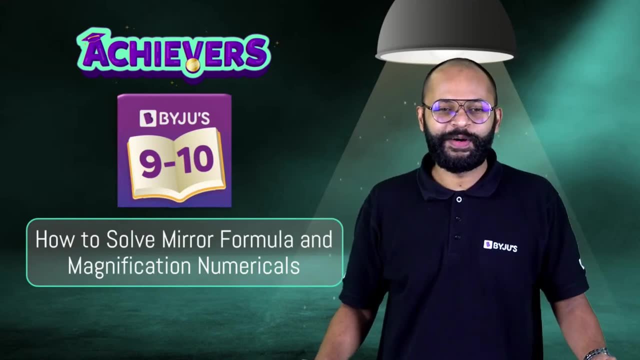 I was going to ask that. perfectly audible and visible. nice, I am good, I am good, it's okay. Arshya, even I was one minute late, it's okay. Adarsh hello, Vivek Raj, Lisa Arush. 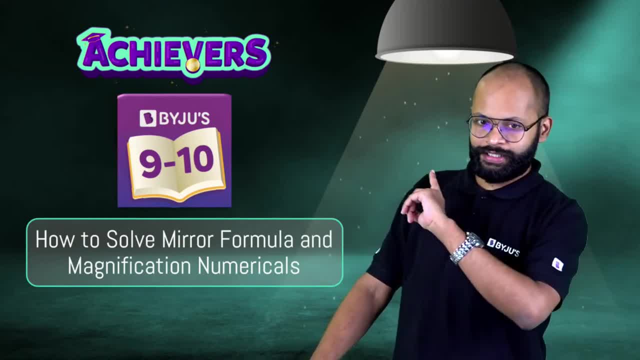 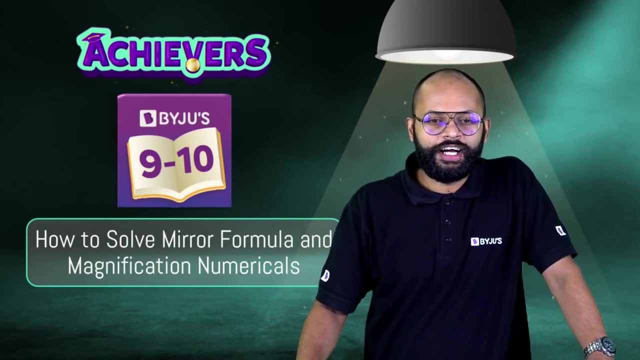 yes, Hello, how many of you have revised this? First of all, tell me that the mirror formula and magnification, Ruchika Anshul Akshat. yes, What we will learn today, Anshul, it's. 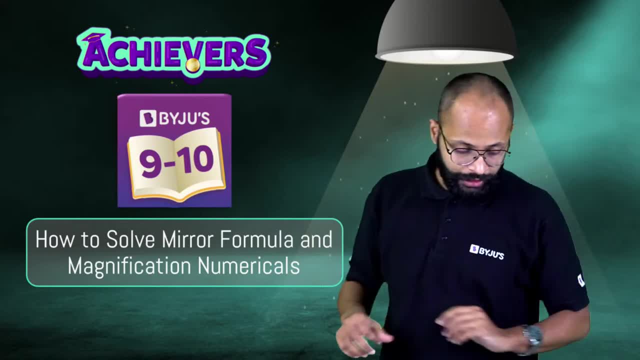 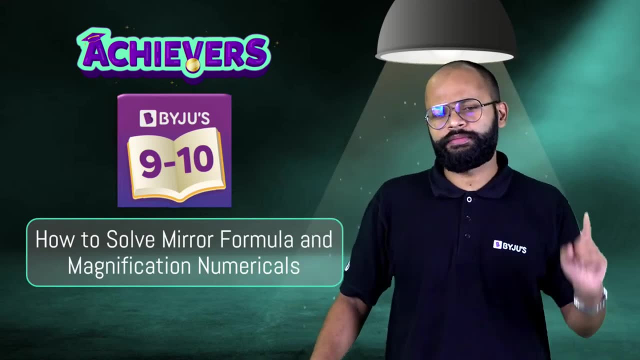 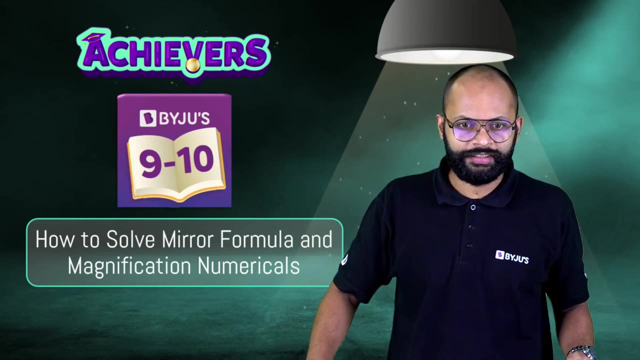 a good question and your answer is here. We will learn about how to solve mirror formula and magnification questions. okay, Ruchika Menti, not today, some day, because I am going to have a discussion and then I will tell you how to solve it. okay, So you guys have 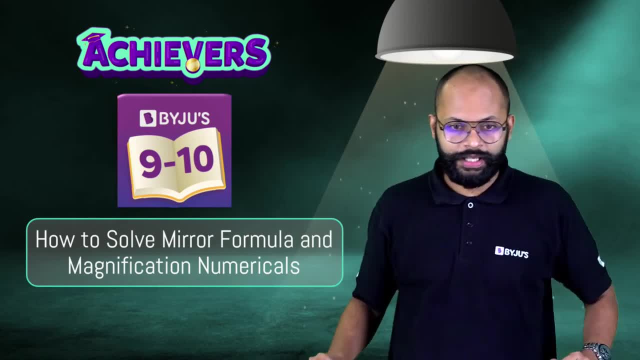 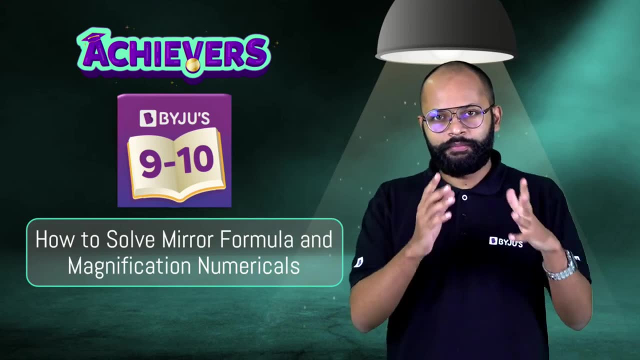 revised it right. Nice, very good, very good. That's oh, Anmol. yes, because in the last session you guys were facing some problems. you know what? This session was not actually planned because, seeing your response, we planned this session impromptu, very, very soon. because, 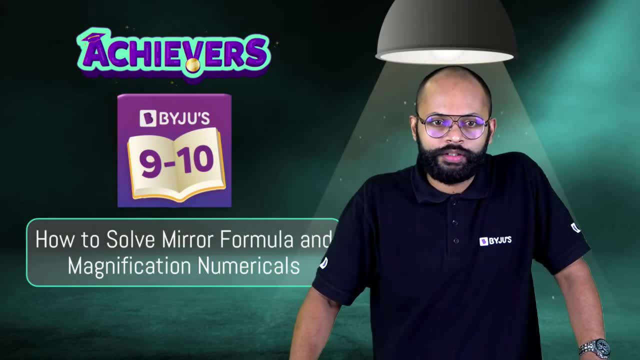 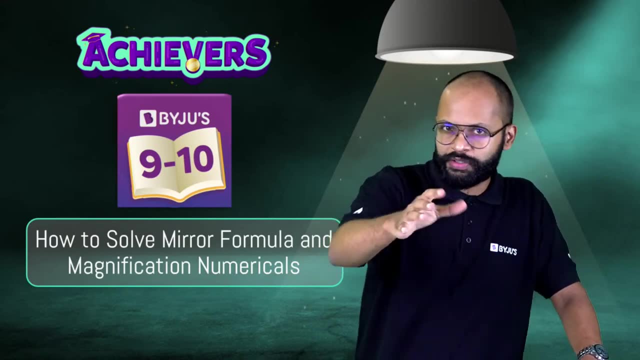 this is quite an important topic and, as you guys- oh, it's okay, Disha, no problem. So, as you guys mentioned, you were facing some problems. I saw your responses, So that's why today we'll have a very quick revision and some questions, because then only a concept gets. 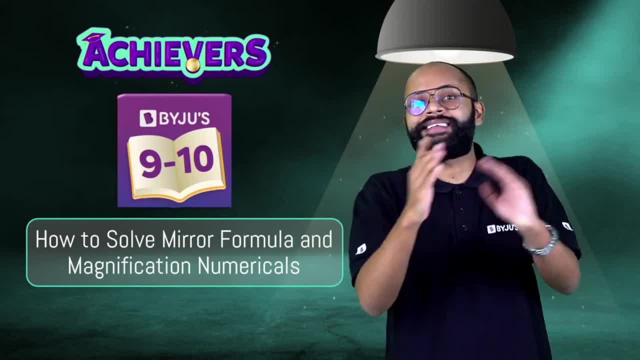 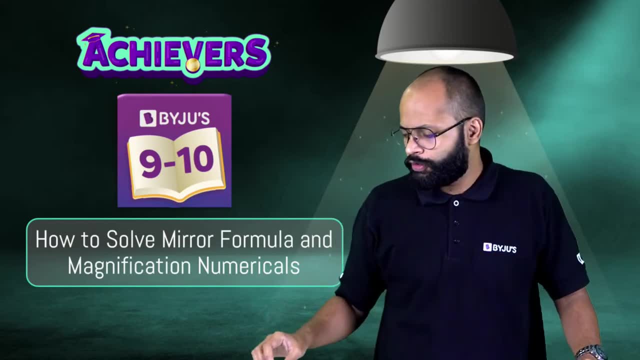 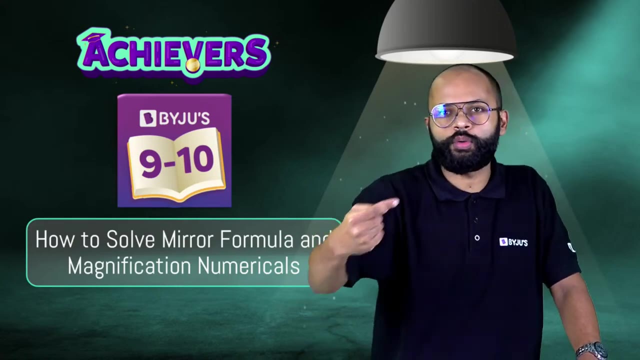 freezed in your head. okay, so today's session is about understanding and application. okay, so let's make it clear and more best book for physics. i would say it's too soon to ask this question. first get the ncrt cleared up and then move on to higher level. and don't worry, we have 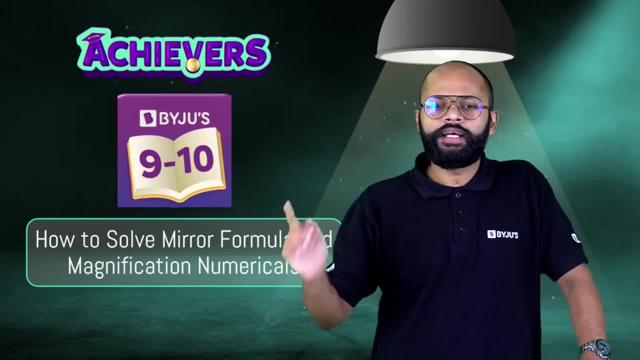 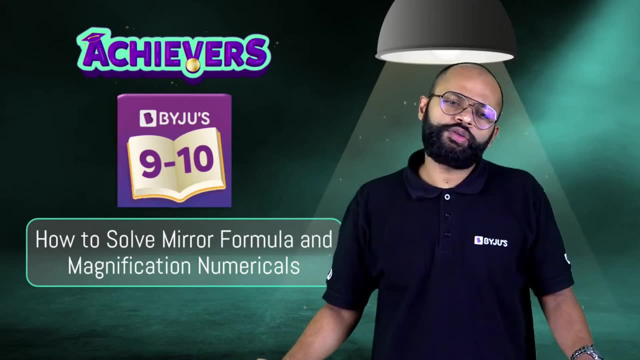 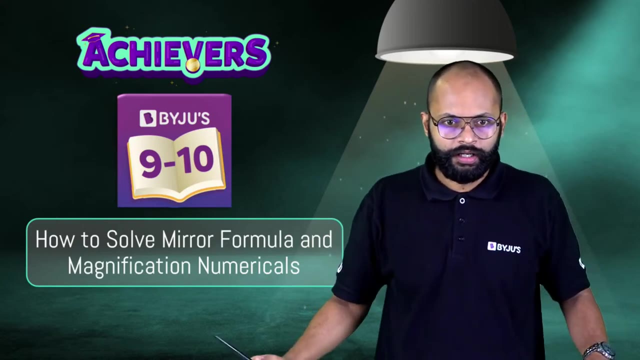 done sessions for this. i have told you multiple books. don't worry, i'll tell you again. like in mirror: formula and magnification. that is the hero of this session. okay, yes, others you can, but sometimes it might go a little above. so right, just, uh, heads up to you. oh, hey, firdaus, yes, 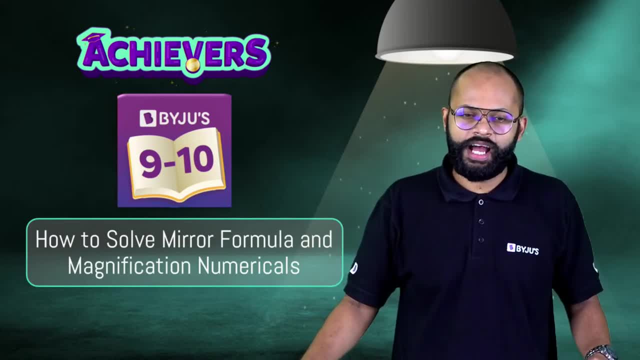 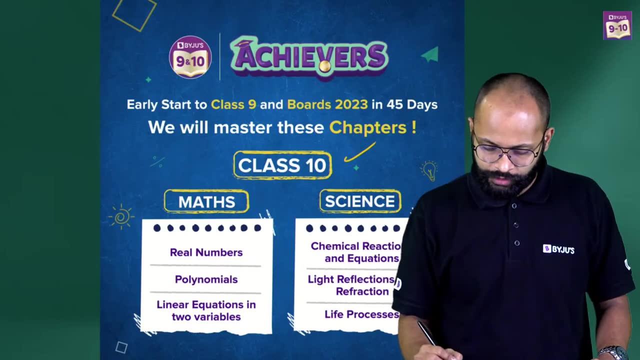 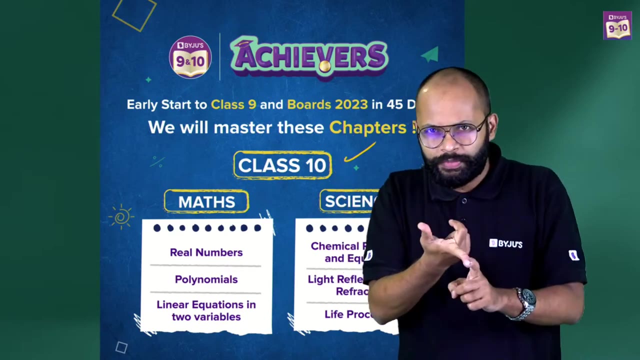 yeah, yeah, this, this we will do see. i told you now there was a 45 days plan. right, there was a 45 days plan for this light reflection. reflection will be completed, completed in this. so here we had given you the whole plan of this right concept, sessions, challenge yourself, questions and exemplar. 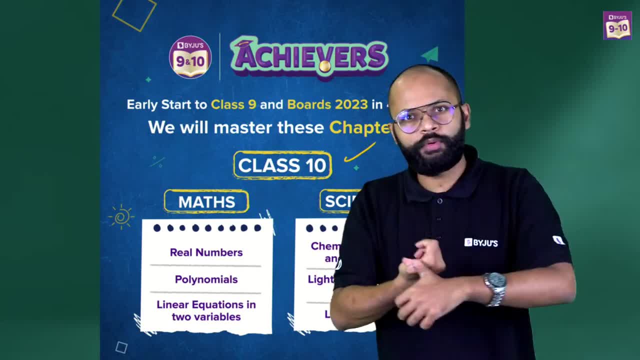 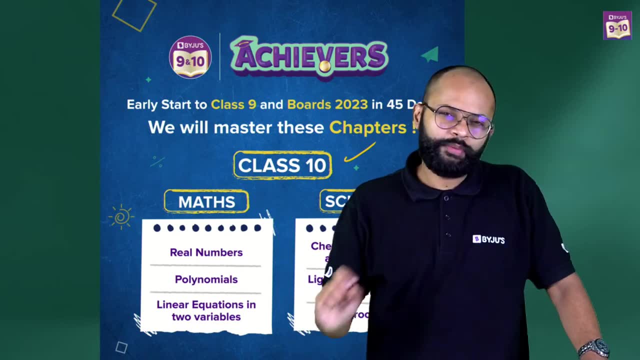 questions. then we have mentee also in that mind map also, and then we have previous year questions. all these things are there. okay, you know pradeep may have a lot of questions. my one problem is this: you get so overwhelmed looking at so many questions gap you. you get scared, so get the. 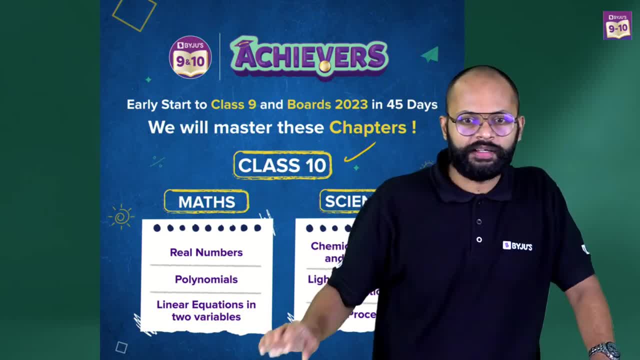 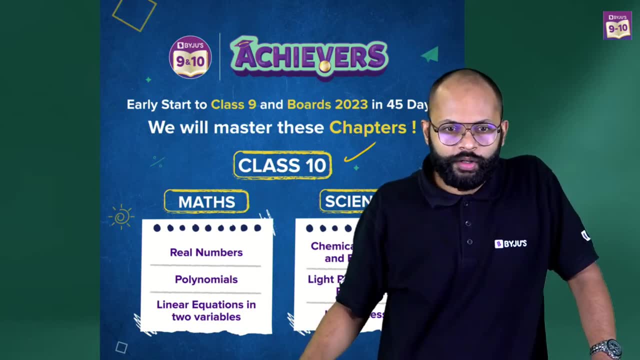 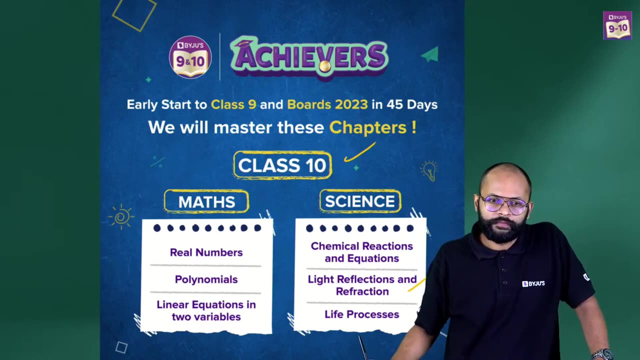 concepts: right. first questions: multiple questions: right, cool, nice, thank you. and that's what mirror formula is right? right, yes, hey, parii, it's okay. hello chetna, hey, uh, birlikte, okay, all right, all right. guys. there was a homework question given to you in the last session. i don't. 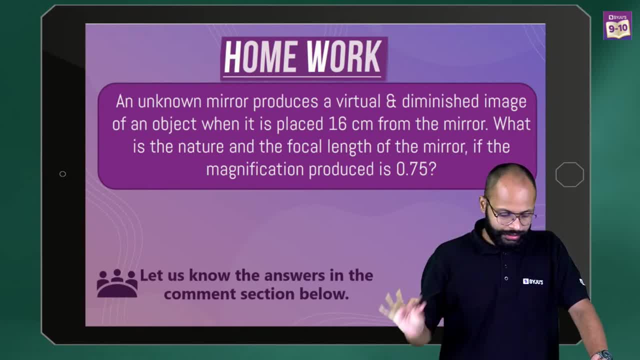 know how many of you have seen this- at least new people, because i have the names of people who try to answer, who gave the answers for this in the comment section. yes, this was the homework question. Now, listen carefully. okay, right. an unknown mirror produces a virtual and diminished image. 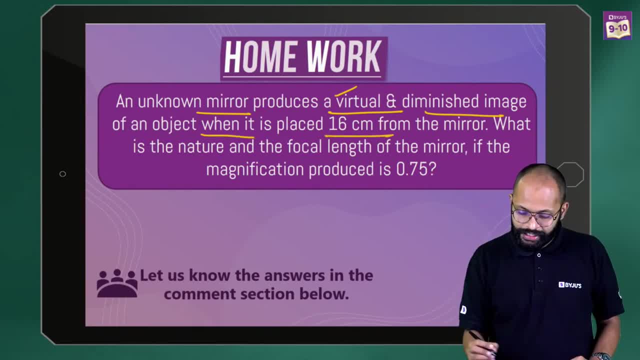 unknown mirror. you don't know what mirror is this right of an object which is placed 16 centimeters from the mirror? what is this Object distance? What is the nature and focal length of the mirror if the magnification produced is 0.75?? 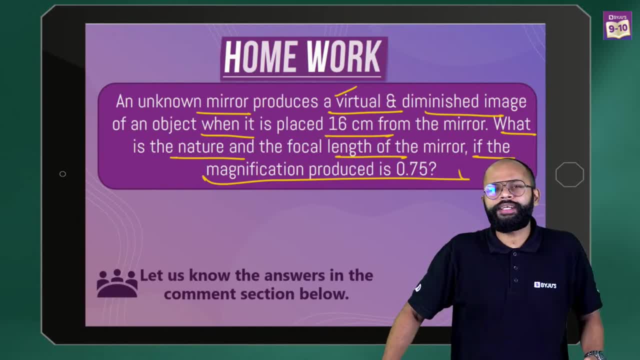 Now tell me something. looking at magnification, what do you understand? Right, Aarush, I'll come about this hypermetropia, metropia. how to do corrections? by the way, it's a focal length, if I tell you. minus it gives you an idea of concave, right? yes? 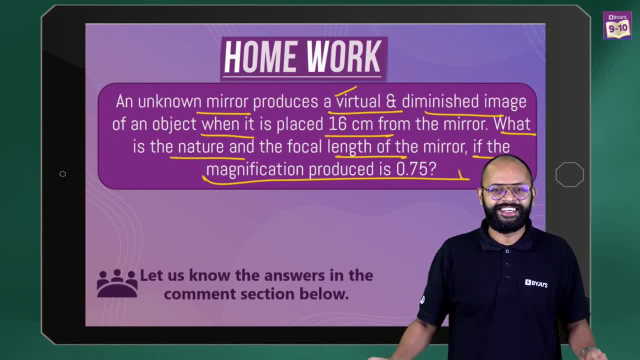 correct. Hey, Aishwarya, yes, I saw. alright, diminished. okay, nice, so you are saying if magnification is 0.75, the image will be diminished? nice, can someone comment about the nature? How much magnified is it? 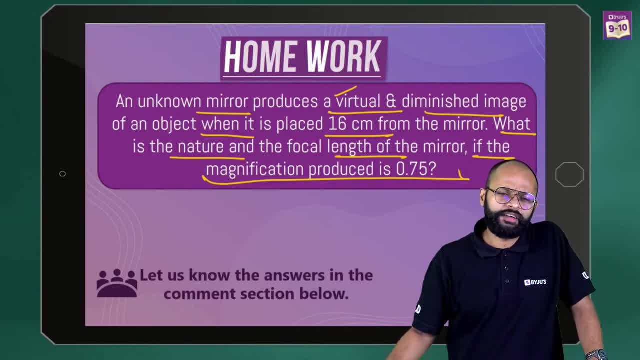 Yes, Anshul, you are right. yeah, Prasad, I have heard about it. nice, Ankita, alright diminished, correct convex, sir. how do you know it's convex? You just told me it's magnification, which is 0.75, how can you say it's convex, right? 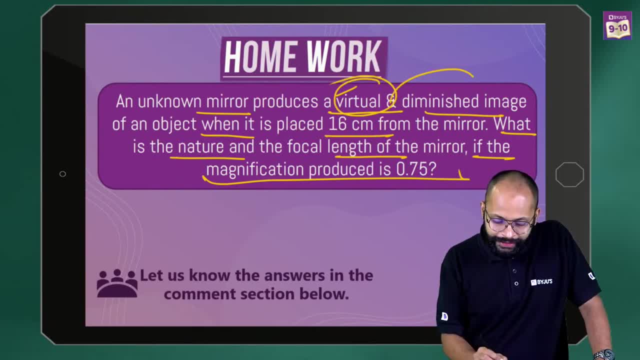 come on virtual, diminished and 0.75, which mirror? can it be a concave mirror? It cannot be a concave mirror, because concave mirror forms virtual image only in one case, when the object is between pole and focus. but that is a magnified image, it's a diminished. 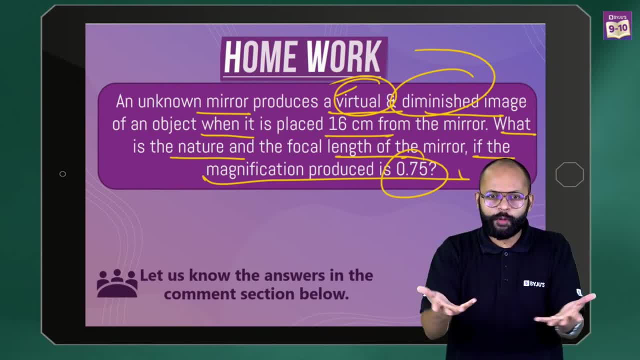 image means it's only a convex mirror. so that's why I'm telling you again and again: right, whenever you are solving numericals, it doesn't matter if you know only the formula right or the only theory. you have to apply both, because when you think logically plus 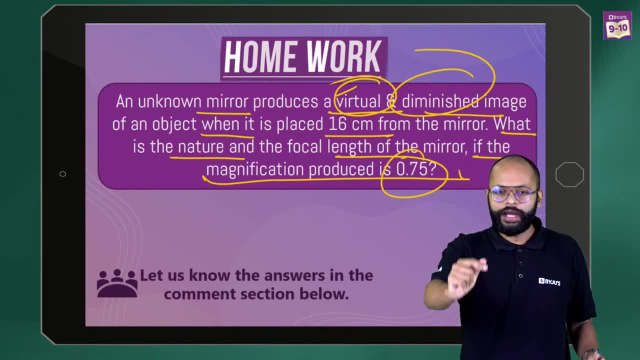 mathematically, then your answer will never be right. Okay, Okay. So that's why you're saying it's wrong and don't worry, today we'll discuss. I will say: today we'll learn how to apply this thing in questions. okay. 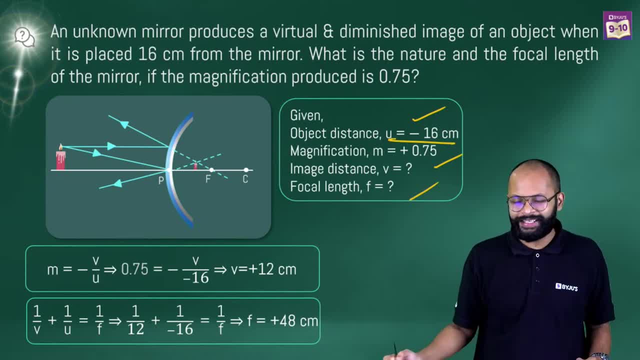 So in simple words, if I give you the formula, object distance u is minus 16y because it is to the left, then m is plus 0.75,. image distance v and f is something you have to find. so m equals minus v upon u. you used the magnification formula, correct. 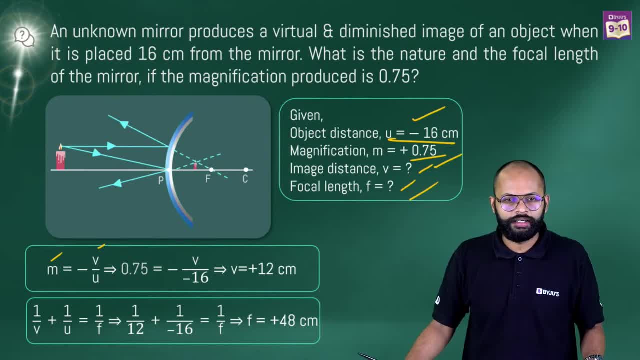 Yes, yes, you're right. yes, Prasad, not a good time with this right, So you have to be more careful. okay, this right? so v equals you will get plus 12, which is which is fine, because the image will be on the. 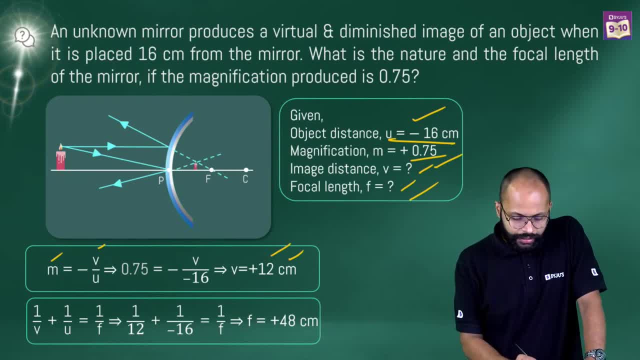 other side of the mirror, on the right, on the right side of the mirror. that's why use the formula: get the answer f equals plus 48 and yes, congratulations, debashish andy, chotabim, shoeb, tavishi, vishal. and yes, i saw your comments. they were step-by-step answers also. so very good guys, very good, a big. 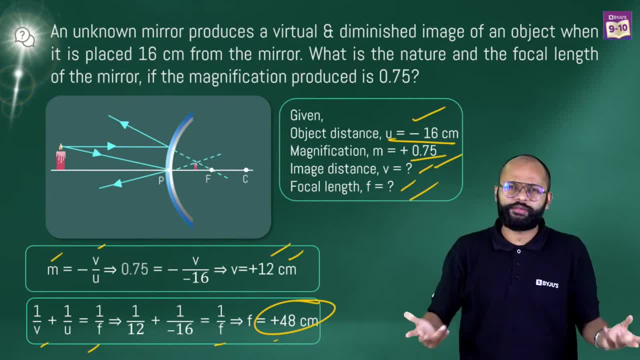 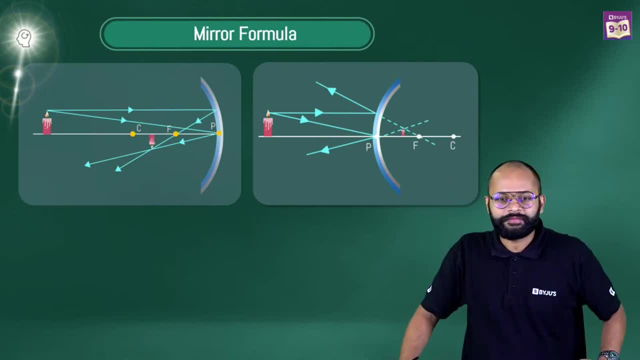 round of applause for you, right, and people who could not solve it. try to solve the next time. and don't worry, let's start. yes, right, yes, 0.75 positive, hey, so mirror formula. first of all, let's get the basics right very fast, very quickly. we'll just clear up the basics. hello, hello, focus. 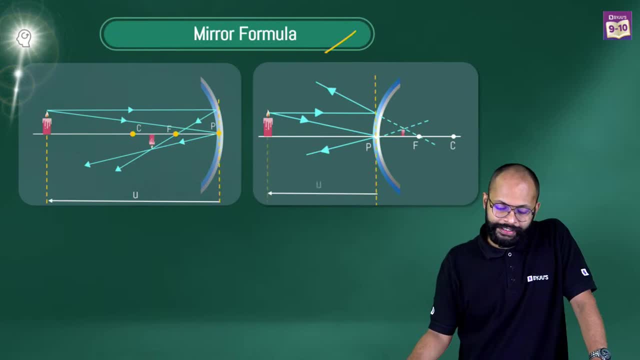 focus, you is the object distance. doesn't matter what mirror is this, you will be the object distance. that is the terminology will follow. ticket: hey, aishi, right, oh, wow, uh, marsh me gamer complicated name. huh, it's okay, rishi. nothing, we haven't missed anything, we're just starting. we just discussed about the homework question. ticket: hey, monisha, so you is. 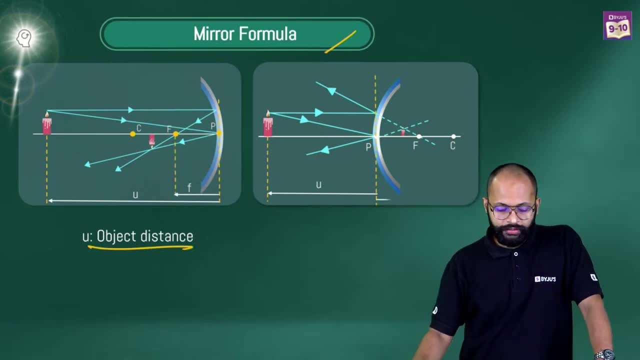 the object distance. fine, simple thing. ticket f is the focal length, right f is the focal length and f is something we'll use again and again for focal length, be it concave, be it convex. ticket plus minus p: we'll talk about this, don't worry, right hey? 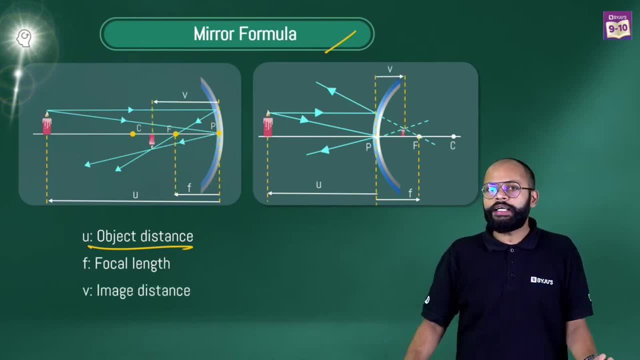 all right. next v v is the image distance. see, whenever you're talking about any question, any question, in mirrors, you will have object, you'll have its distance. you will have object. uh, you'll have the focal length, you'll have the image distance. okay, these are few things which will 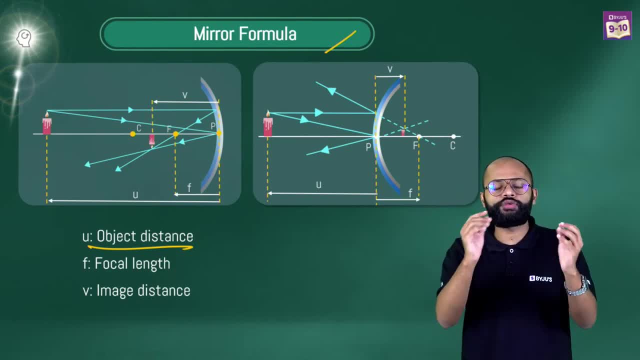 come repeatedly in a lot of questions, so that's why it's very important that you should know what is the meaning of u, v and f and you should know what is the meaning of u, v and f, and you should understand the meaning of u, v and f and i think you know. okay, give me a good thumbs up if you know. 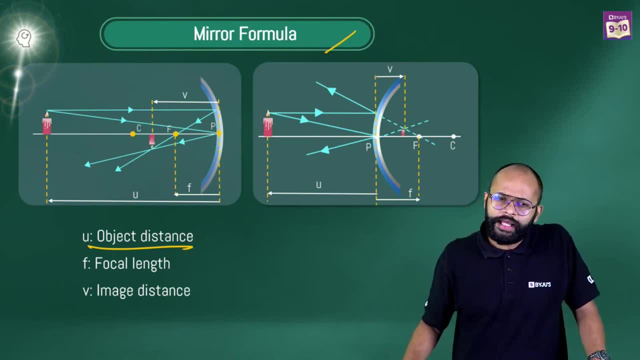 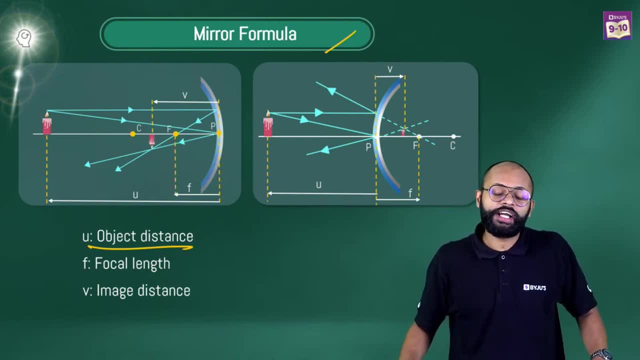 Wow, very good. Ishika is always virtual, I think you are trying to ask: is you always real? is the object always real? I would say right now I won't comment on this because we have virtual object concept also, but later, not today, focus Monisha: yes, alright, yes. 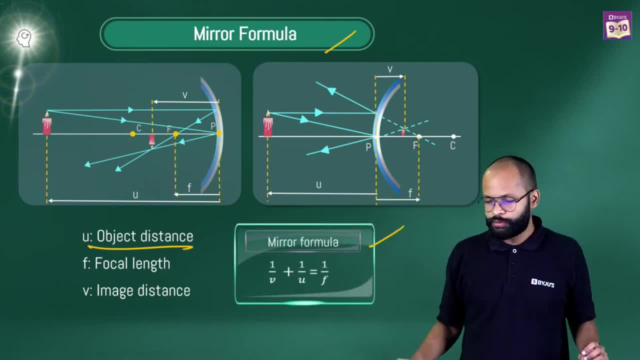 come on, and this is the formula we are going to use now. I want to ask you one thing: how many of you tried to derive this formula? I am not going to derive it today also. I am just asking you how many of you tried to derive it and how many of you feel that. 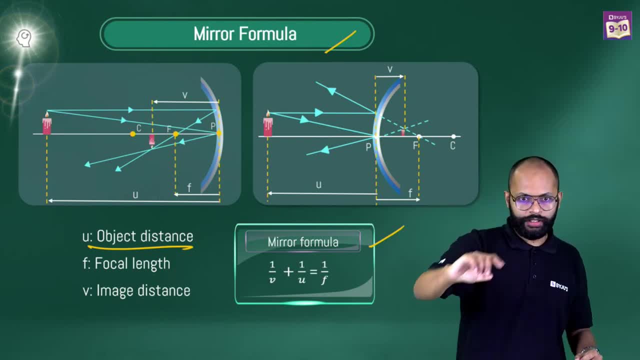 you want to learn how to derive this formula, and this is important. give me an idea over there. Anshul says he knows nice, Okay, nice, it's good that you are studying while you are in the form. Ishika says she. 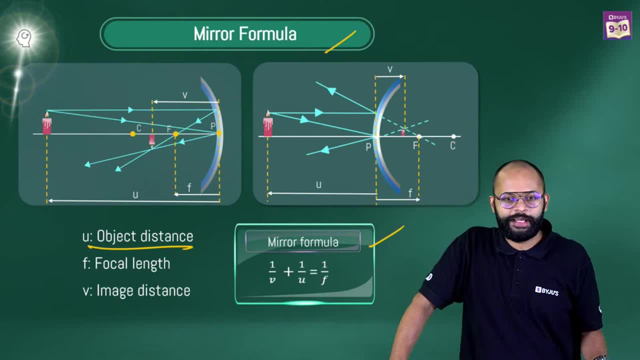 wants to learn Vivek Raj- good kids gaming. I know I want to learn. already done, Adisha, you are a senior. you have already done Ishika. the reason Tavishi did want to learn, learn. 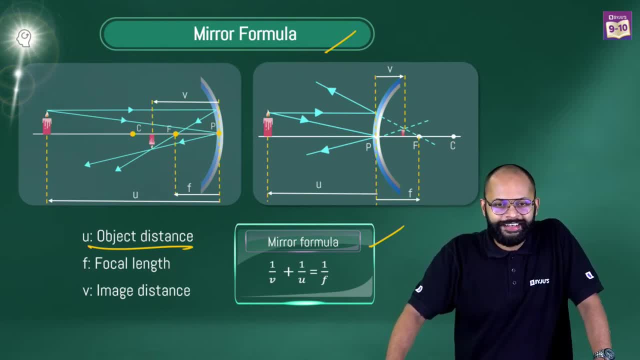 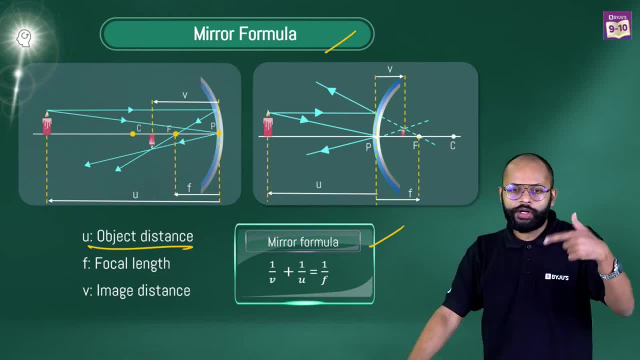 but soon, okay, alright. so that's why I wanted to ask you that: are you facing problem in that? because if you are, we will share the derivation with you. I will make a video and share it with you, okay, alright, alright, alright, okay, let's move forward. sign convention. 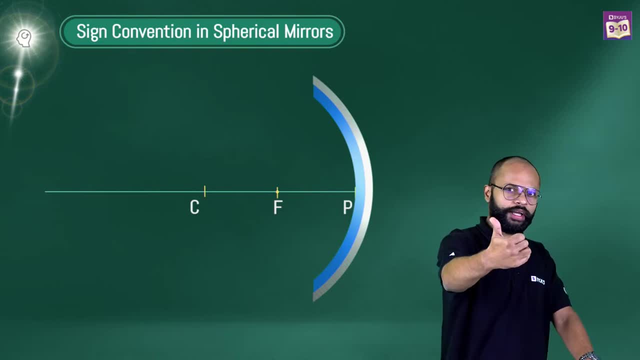 spherical mirrors. okay, I will just keep naming and you keep telling me is it positive or negative. and people who are facing problem. I will just keep naming and you keep telling me is it positive or negative. and people who are facing problem. right, who are facing? 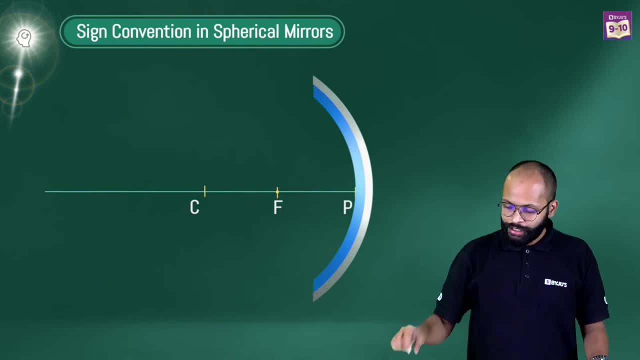 problem, then let me know in the chat. can you tell me what about left? left is positive or negative? oh, yeah, yeah, scientific, it's not there. negative, negative anyone, anyone in the chat? no, no, it's not positive, it's negative. right, it's negative, okay, okay. 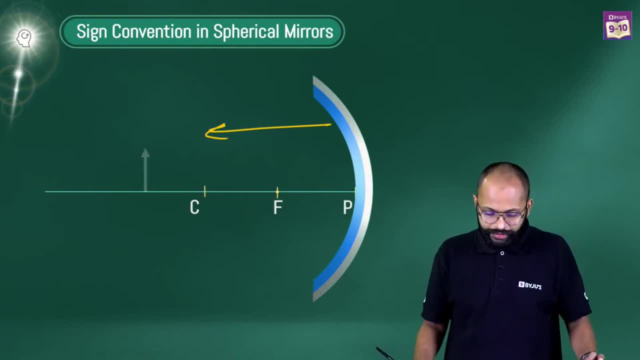 correct. so left is negative. why is it negative? because object is to the left. let's say object is to the left. so we go with Cartesian coordinate system, in which plus x minus x, plus y minus y, right? so this is what I am saying. yes, correct, correct, Ishika you. 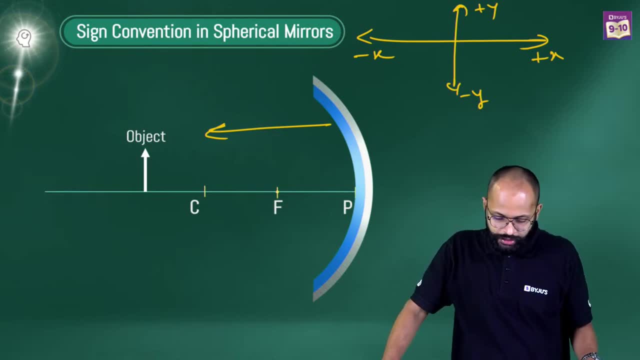 are right. yes, very good. okay, if you answered left, which means right, I don't think I need to do anything else. this up means this height of object. will it be plus h or minus h? tell me no, no, gamer, I won't say that positive right, because it is above the principal axis. 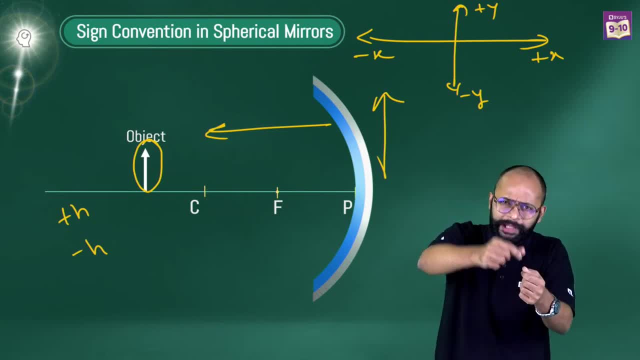 if anything. if you are measuring above the principal axis, you are going in plus y direction. no, that's why it's going to be positive, correct? Yes, Parvati, it's actually there, if you ask me. so this is what. this is the coordinate. 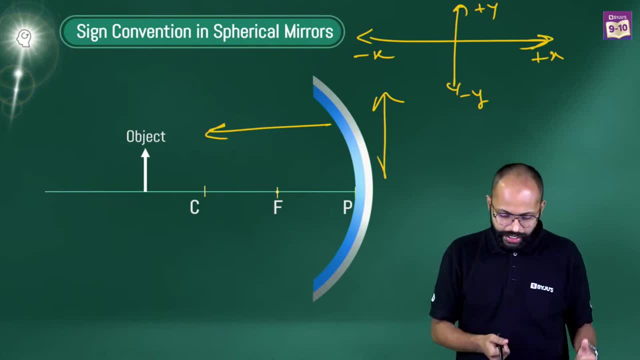 axis in maths: right plus x minus x, plus y minus y. so you have taken pole as your origin. this o becomes your p. that's a very, very, I would say, easy kind of relation that you can make so very quickly. if you have an object, you have an image, right, you have. 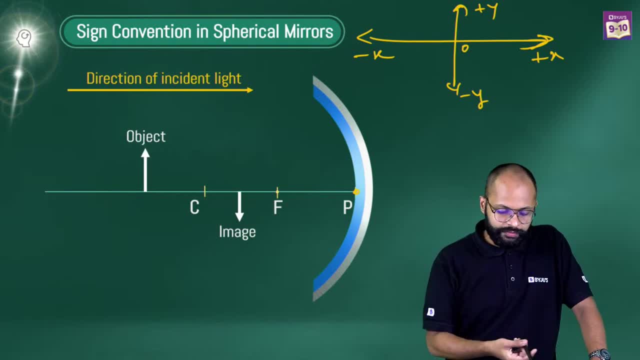 the direction of incident light. the reason I am showing you incident light is because a lot of students get confused in this. okay, Sir, what if? what if the light was coming from the right, then what? then what? so normally it doesn't happen, but, let's say, any competitive exam tries to confuse you in this manner. 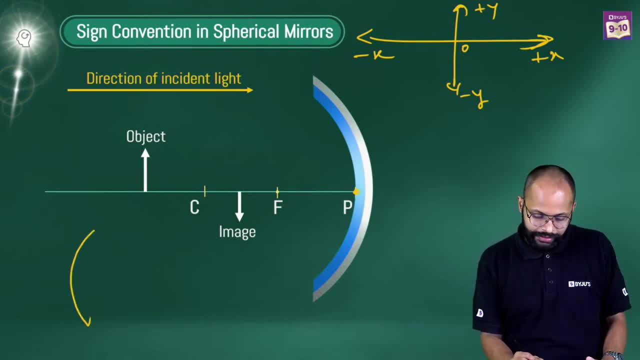 okay, you know, let's say: the mirror is not like this, mirror is like this. if mirror is like this, then then. so if you go in the direction of incident light- I am saying this too- we have learned: plus x to the right is plus, left is minus, up is minus. so this: 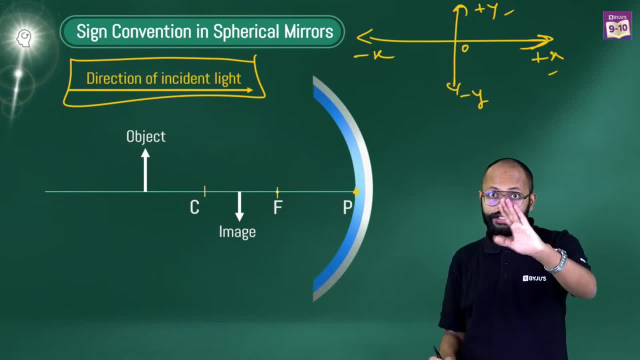 is plus, down is minus. so if the mirror is turned like this, right so we are actually taking positive to the measurements taken in the direction of incident light. so what do I mean? if you are going right, you are actually going in the direction of incident. 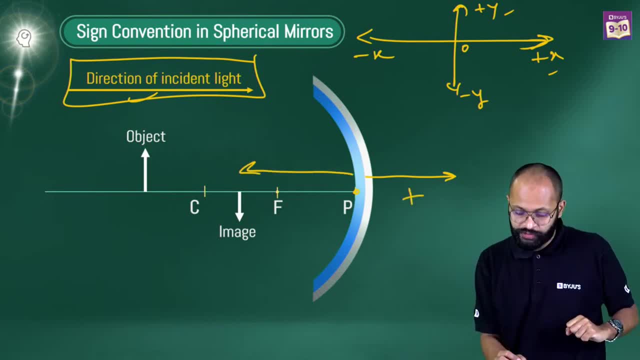 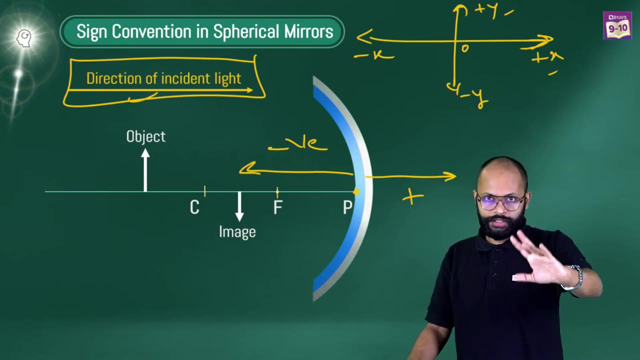 light means plus. if you are going to the left, you are actually going opposite to the direction of incident. light means negative, so got it right. so that's why I am trying to explain Something over here which is a confusion which might come in future. okay, I am just 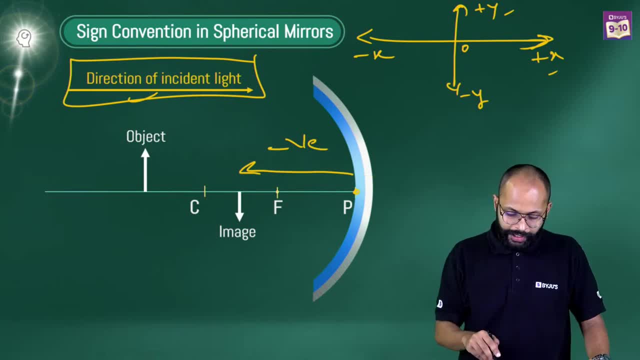 anticipating. that's why I am telling you: okay, alright, plus minus. this is very important, right? don't be confused. don't be confused, nice, okay, no, no, no, Ishika up will still be positive right. up and down will not change, don't worry about that, only left and right. 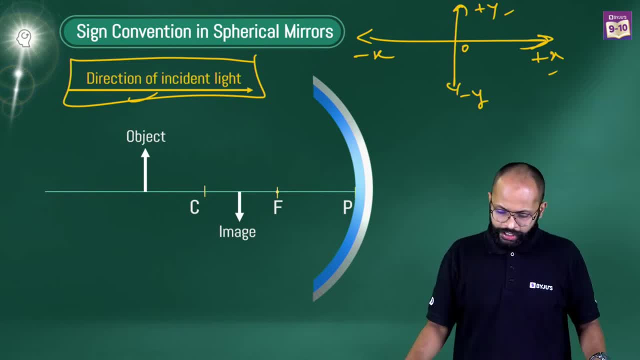 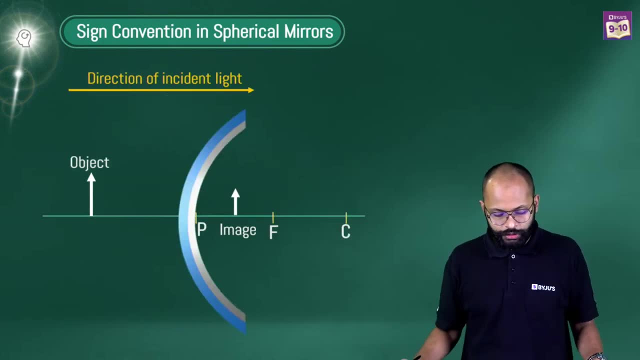 will change. okay, don't worry. nice, very good, very good guys. So left is negative, right is positive, up is positive and down is negative. this is something which you guys know. now, if I change the mirror, if I make the mirror as convex, 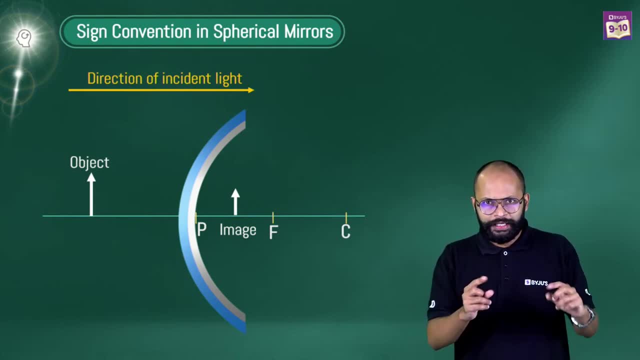 mirror. will it matter? tell me, will it matter? left will still be negative, right will still be positive, up will still be positive and down will still be negative, right, okay, it's okay, it's okay. so that's why we are here, no. 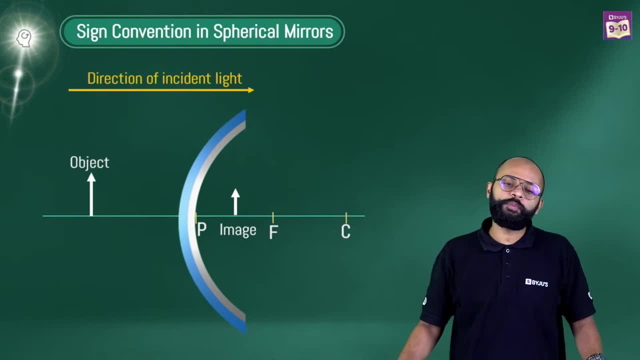 Up and down. Parvati is used, they will give you height of object and they will ask you height of image. or they will give you height of object and image. so if the object is up and let's say, the image is inverted, so image height is like this, so you say that image. 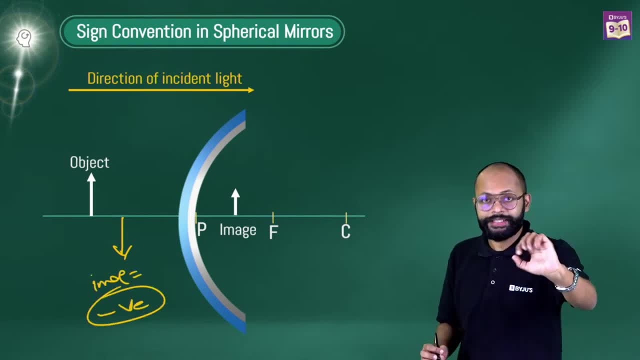 is negative. okay, height of image is negative. that's how it comes. okay, yes, no change. very good, I am sure no change will happen. it doesn't matter. The sign convention remains the same right, it remains the same. so, positive, negative, 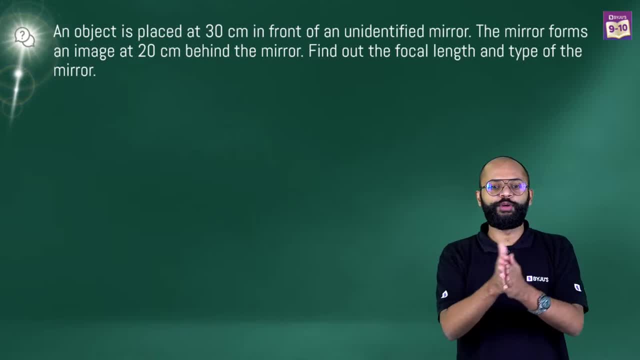 negative, positive, still the same. okay, if you know that, if you understand that, let's jump to a question. let's be real and let's apply the knowledge. okay, first question in front of you, let's solve it. and it's okay if you face problem, because 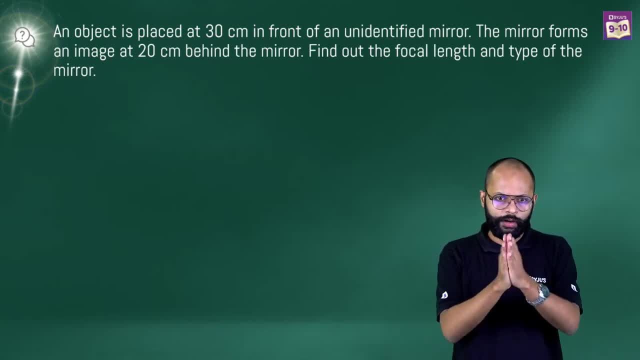 you know what? I will be glad that I can help you, okay, alright, come on. come on, guys, come on. An object is placed at 30 centimeters in front of you. Okay, An object is placed in front of an unidentified mirror. yes, Parvati, your doubts will be. 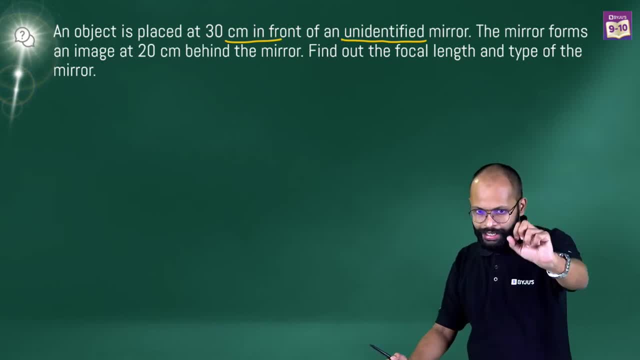 clear. don't worry, focus on the questions, because all the doubts you are asking, no, they will come in the question itself. right, so apply the knowledge and you will understand more. okay, right, so an object is placed at 30 centimeters in front of an unidentified 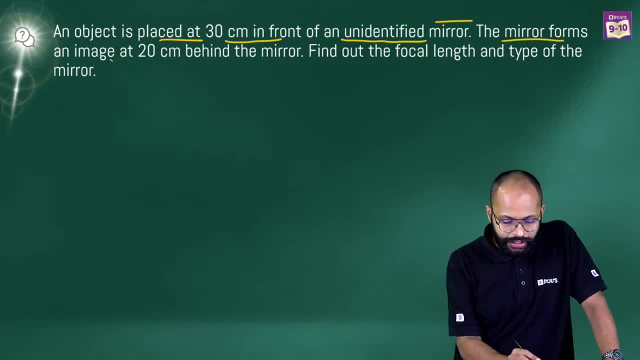 mirror. you don't know what mirror is this? okay, the mirror forms an image. at 20 centimeters behind the mirror, find out the focal length and type of the mirror. okay, so what did I tell you? before jumping on to the formula, read the question. think. what is the question. 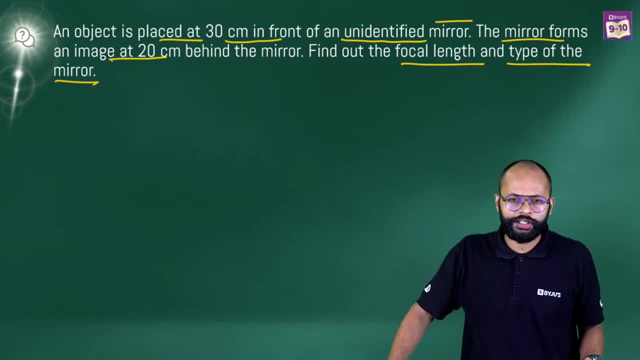 trying to tell you: right, come on, come on, focus, focus, guys. right, you have been given the object distance. this is 30 centimeters in front of an unknown mirror. I don't know what mirror is this? now mirror is forming an image at 20 centimeters behind the mirror. 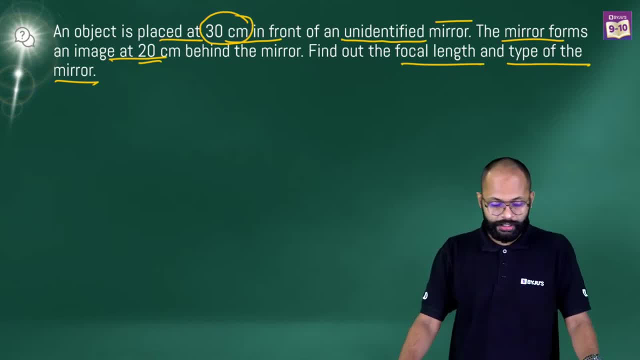 behind the mirror right It is forming an image 20 cm behind the mirror, okay, And you have to find the focal length. Fine, Yes, Okay, Tavishi, Nice, Alright, Alright, Okay, Yes, Alright. See, let's solve it, and then I'll comment more. 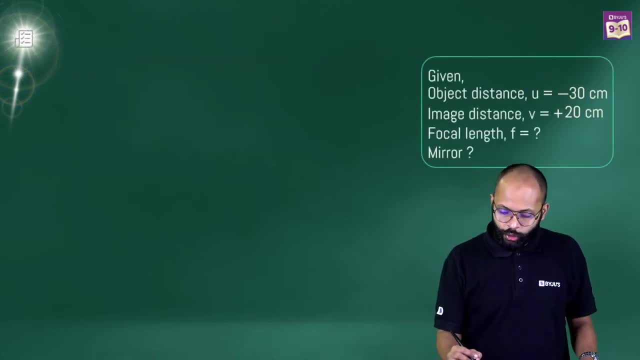 Nice, Nice, Amulu, Very good, So U is minus 30.. Sir, why is U minus 30?? See, even if I don't know what mirror is this, That's why I'm drawing a box, Okay. 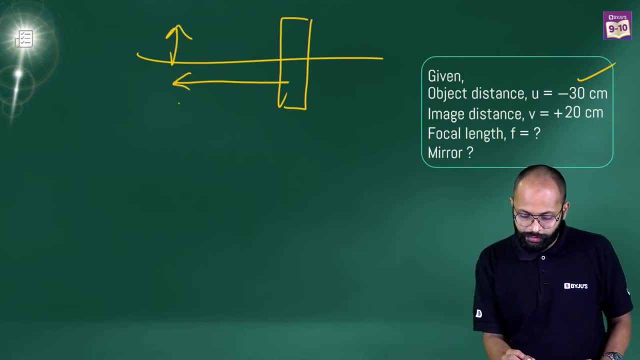 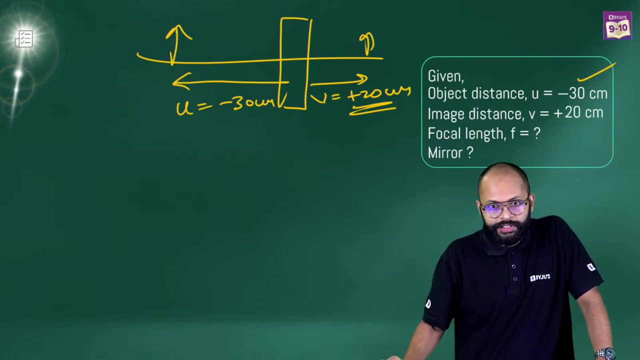 U is in front means this is to the left, means U is minus of 30 cm. It is given to you Image is inside or behind the mirror. So this is V. V is going to be plus 20 cm. It is going to be inside. That's why it is plus right To the right. Okay. 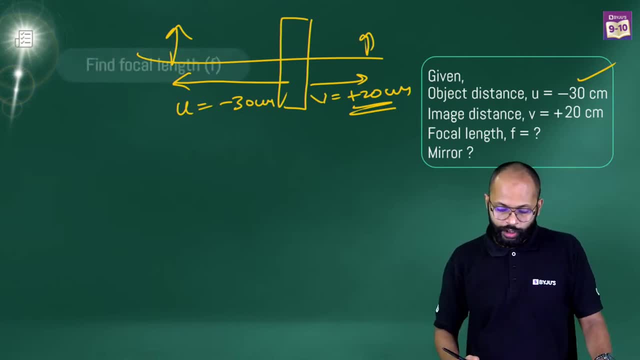 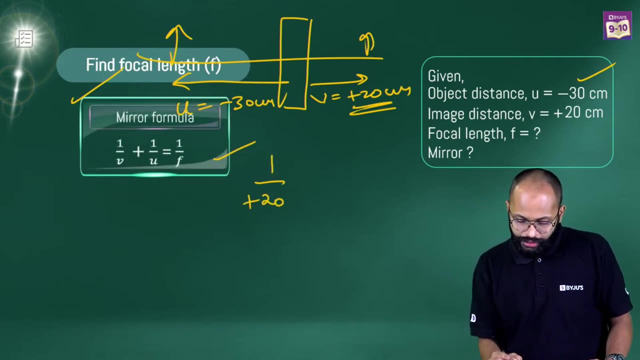 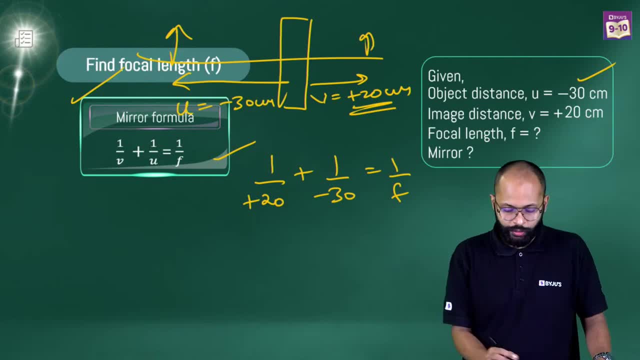 Equals 1 upon F. F is something which you have to find. You will take the LCM 60. And you know what: 3 minus 2. 1 by 60. So F is going to be plus 60. Right. 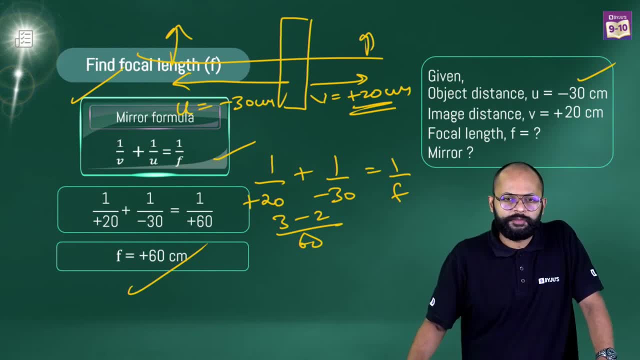 So F will be plus 60 cm. Yeah, Prasad, Please, Please, Last doubt, Right, Come on, Come on, Yes, Yes, Alright, You got 60 cm. Fine, And it is coming out to be positive. Right, It is coming out to be positive. 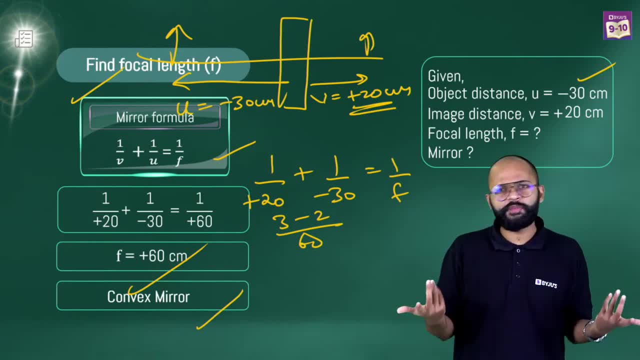 Means it is a convex mirror. Right Means it is a convex mirror. Correct, That's true, Right Got it. Nice, Nice, Very good. Nisha Gets Gaming. Aditi, Amulu And Prasad. you are asking a doubt? Okay, Tavishi, Very good, Nice, Got it. 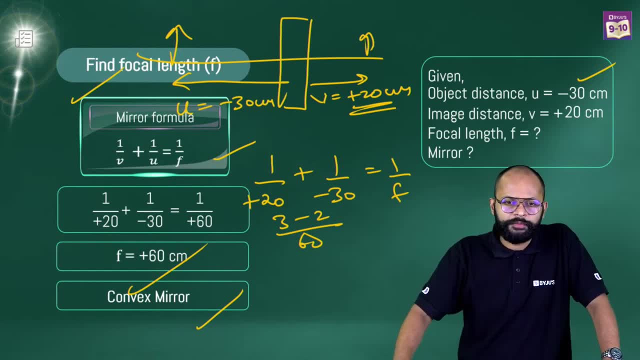 Fine, Alright, Alright, Okay, Let's move forward then. Okay, Okay, Anyone is having this doubt, Sir, if it was plus 60, how can we say it is convex mirror Anyone? Because, see, today's my motive is: Yeah, Andy, That was the intent. 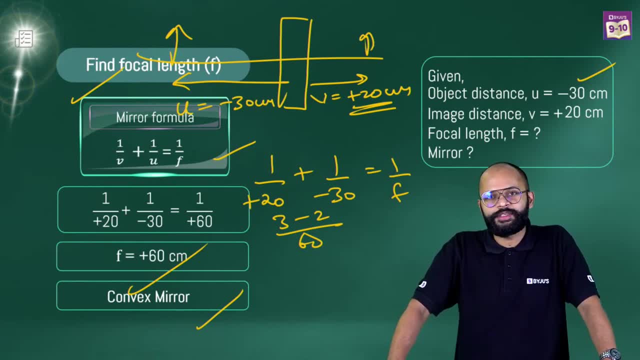 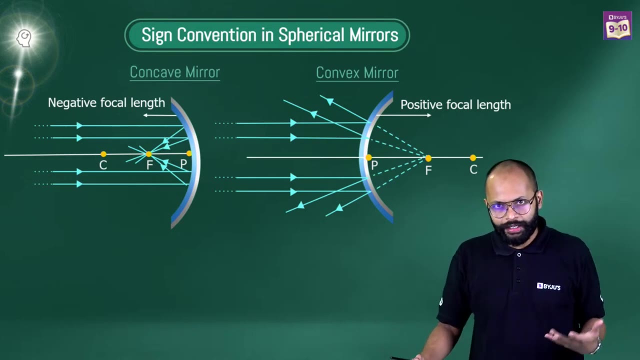 See, I am not very good in these things. My team just gives me ideas about this, So, alright, I just know teaching man And nothing else, Right, Yes, No, Right, Okay. The reason I ask this to you is because you should also be aware that tomorrow, 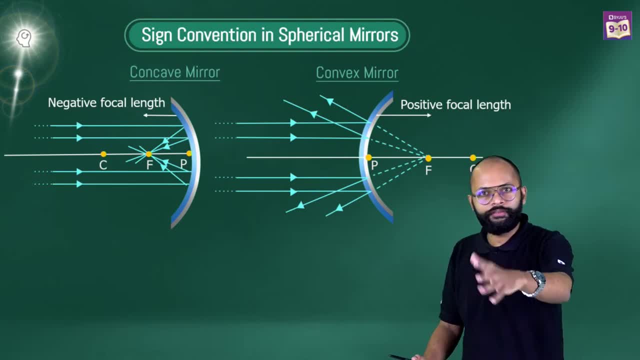 if someone tells you that mirror is concave or it is convex, you should get this idea that, oh, if it is concave, the focal length will be negative, If it is convex, it will be positive. But why, You can ask me. That's why I am telling this to you. Yes, Nice Pratibha. 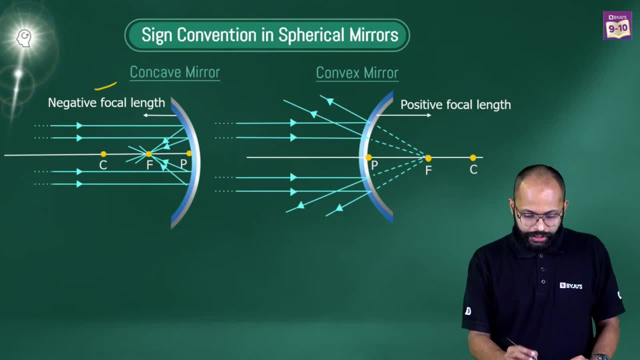 I answered this question only. So concave mirror: what happens If all the parallel rays fall on the mirror? they reflect and really meet at a point. This point is what we call as focus. So focus for a concave mirror is to the left. 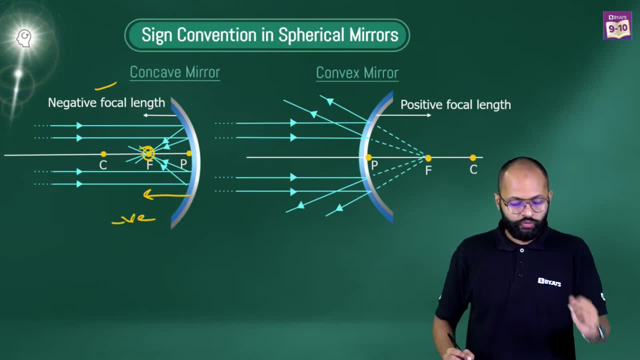 If you think it is to the left? no, It will be negative. So focal length of concave mirror is negative For a convex mirror. when all the parallel rays strike the mirror, they get diverged Means. if you think on the left side, they will never meet. No, So what is happening? 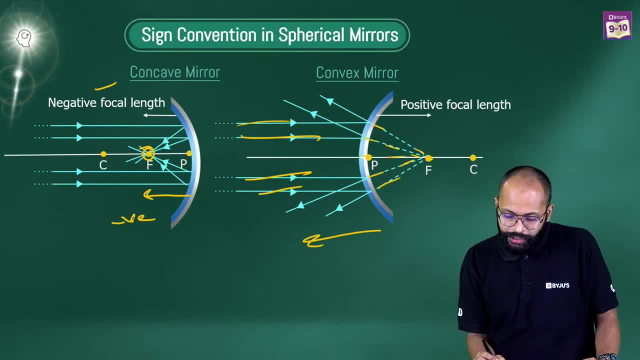 We trace them behind the mirror and they appear to be coming from this point, which we call as the focus. Focus for convex mirror. That's why it is to the right, That's why it is positive. So got it Right. Nice, Deonu. 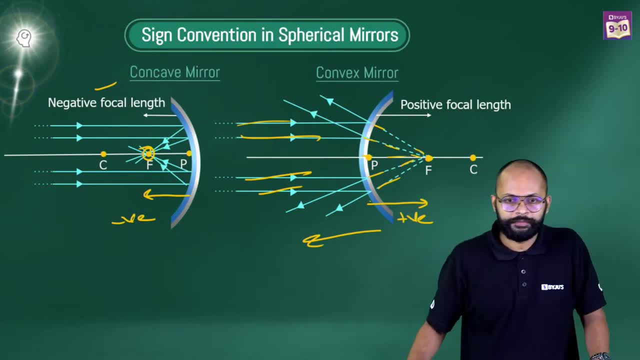 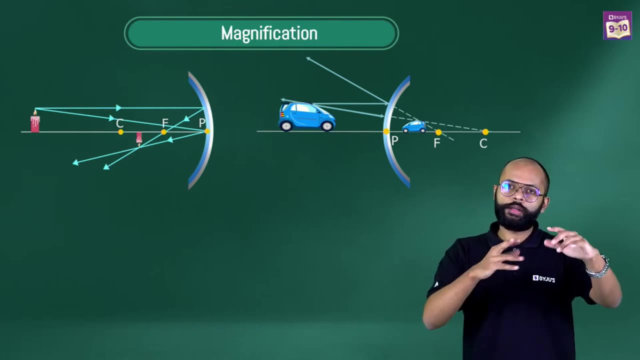 Maybe I am pronouncing it wrong. Hey, right, Correct, Got this. Fine, This is important, guys. This is important, Nice, Alright, Great, Let's go Now. let's talk about magnification. See, we have talked about object distance, image distance and focal length for both the mirrors. 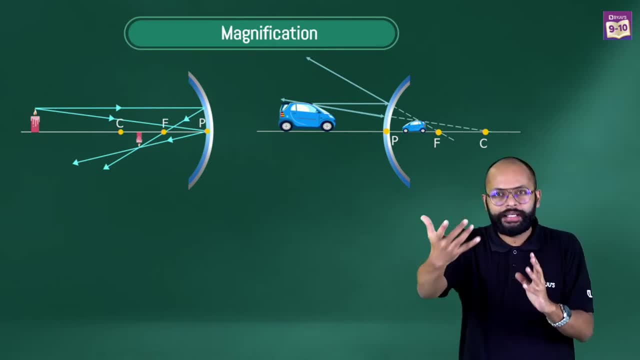 Now you know what You have seen. images are either magnified or diminished, Right? So that's where the magnification comes into picture. Alright, Guys, focus. You can have a personal chat, It's okay, Right? So in concave mirror. you see, here we have a diminished image, Right? 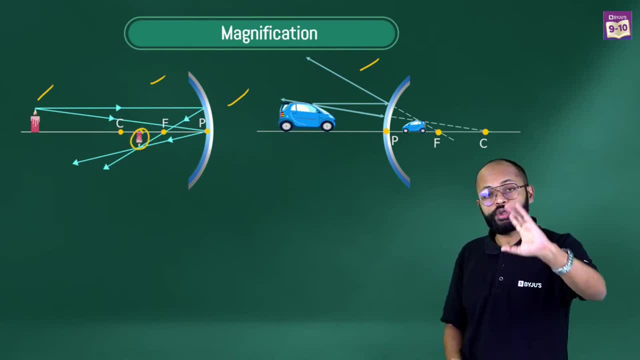 A diminished and inverted image. Right, It's also a real image, Fine, In a convex mirror you have a diminished image, You have a virtual image and you have an erect image. Right, Correct, Right, Got it Alright. 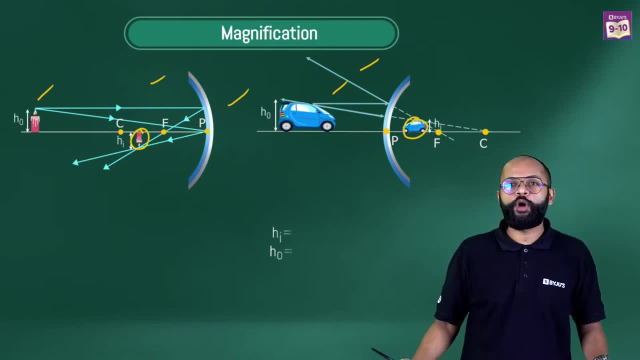 So height of object upon height, Sorry, Height of image upon height of object. What is magnification? It is height of image upon height of object. See why are we doing this? What is the meaning of magnification? How much bigger it has become, Right. 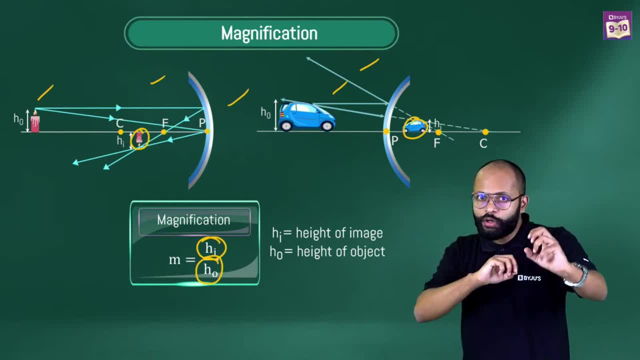 How much big. It's the comparison. It's the ratio. So the ratio of the size of image upon the size of object Means the height of image upon height of object. This ratio is what we call as magnification. Got it? 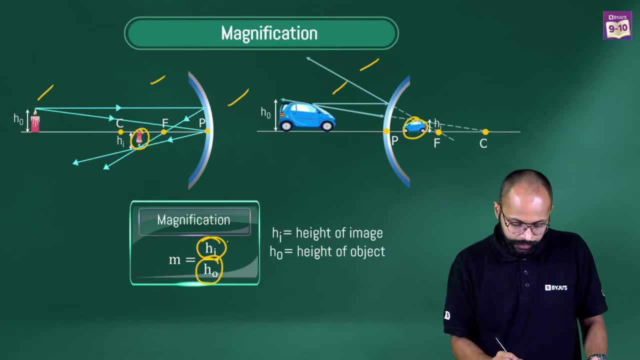 So basic starts from here. The basic starts from this: HI upon HO, That is magnification, Right, Alright, So got this Easy, Okay. So if you got this much Now, if it is positive, means image is upright. 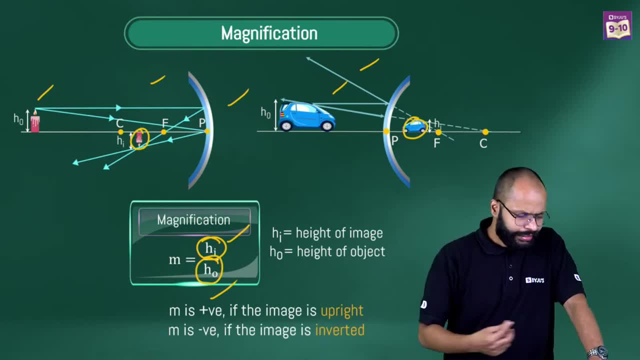 And if it is negative means image is inverted. Do you really need to remember this? Can someone tell me, do you need to remember this thing, Or you understand this- Why it is positive means it is upright And why it is negative means it is inverted? 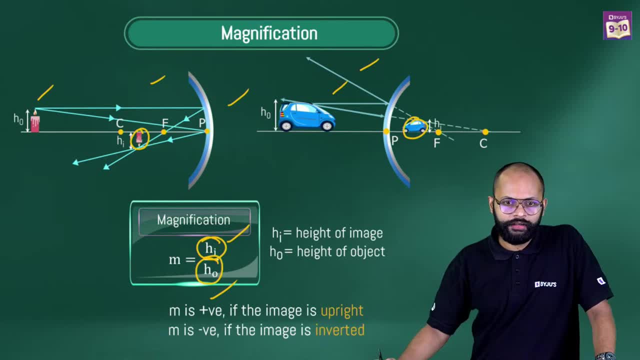 Right, Correct, Got it Nice. Upright, Upright. See what is happening in upright. Image is also erect. Object is also erect Means: HI is going to be positive, HO is going to be positive Means. plus upon plus will be plus only. 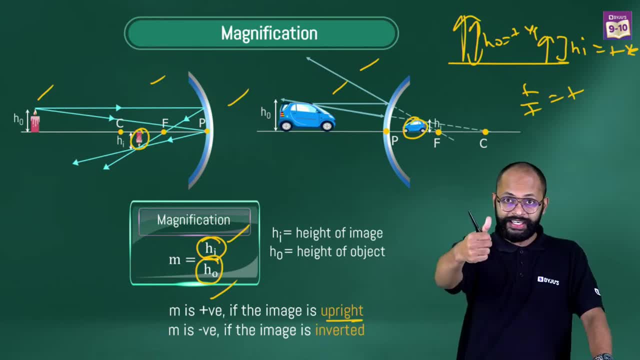 No, Right, Right Correct. Similarly, if it is inverted means image is negative, Object is positive Means minus upon plus will be negative. That's why negative is inverted and positive is upright, Got it. That's why I am saying yes and sure it can be. 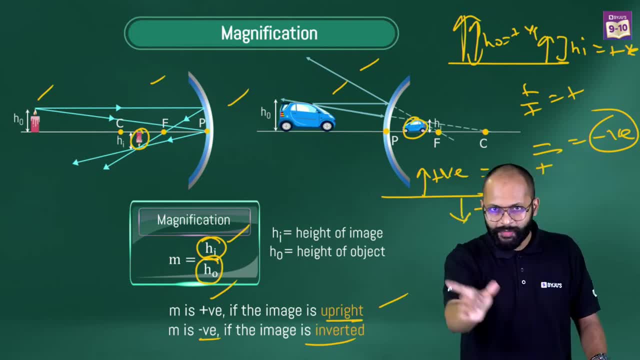 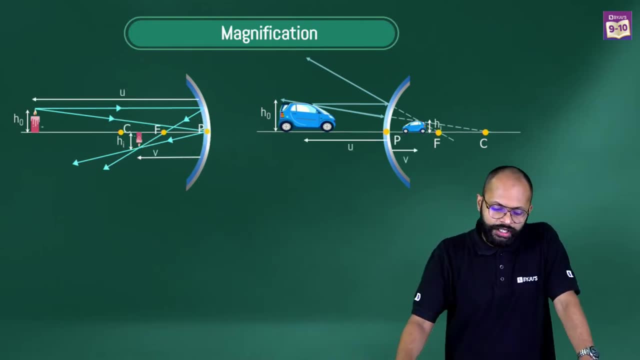 Understood. See, I am trying to cover as many points as possible in this small concept, So that's why I am saying focus Alright, Got it Important, Got it So magnification. one more formula that comes is minus V upon U. 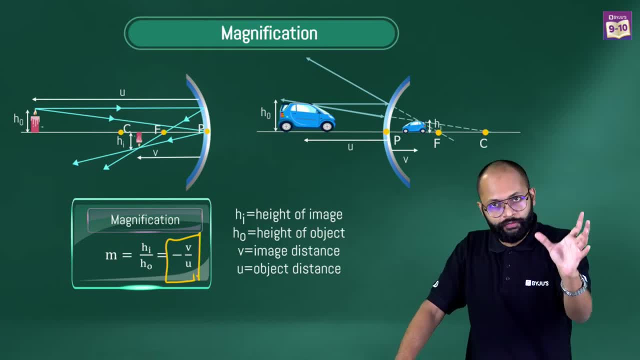 And if you know the derivation of the mirror formula, which means you can also find this. And don't worry, We'll see, We'll make it happen Because of sign convention. Right, Yeah, Correct, So minus V upon U. 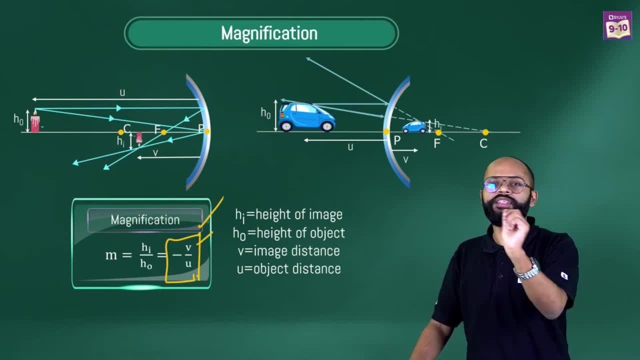 So M in mirrors, spherical mirrors, will be minus V upon U, That is, minus of image distance upon object distance. Okay, Alright. Yes, No, Neo, It's not possible. Real image is there at center of curvature, but not virtual. 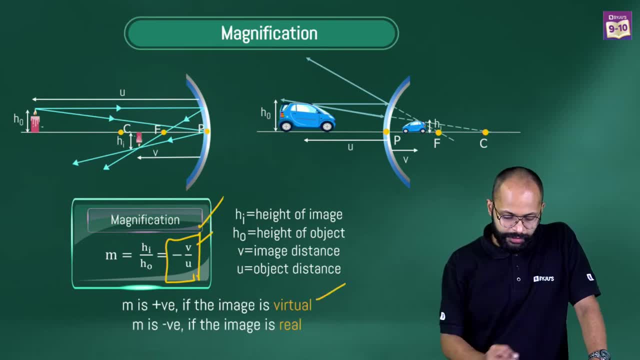 Okay, Fine, Okay, So if M is positive, image is virtual, If M is negative, Then the image is real. Got it Fine When object is placed at F, Because, Nisha, if you retrace them behind the mirror. 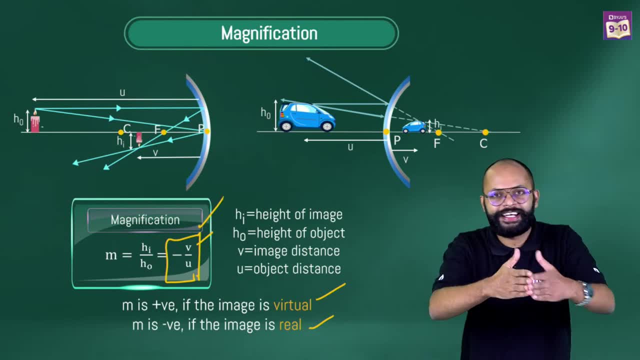 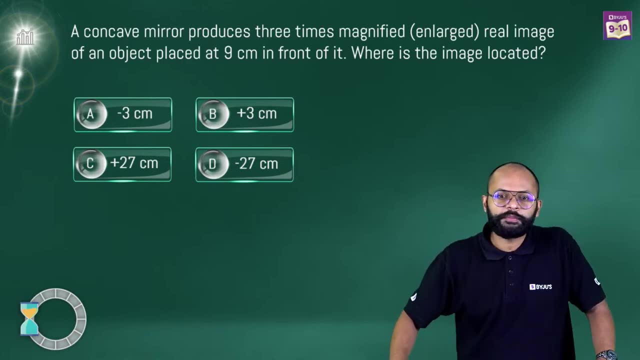 No, They will still be parallel. They won't become converging inside the mirror. That's why. So okay, Here's a poll question for all of you. Come on. Come on, A poll question, Right, Ishikari? it's possible if your object is inverted. 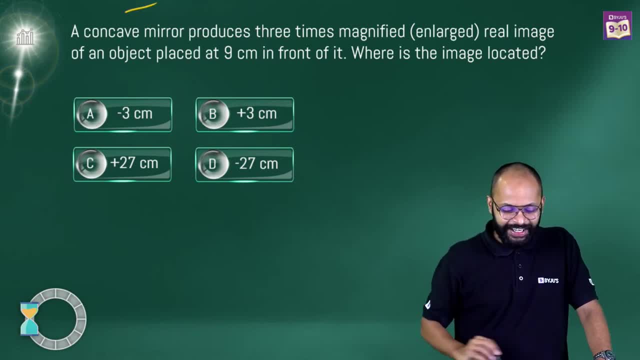 Image will become Real and direct. Alright, Okay, A concave mirror produces three times magnified, So this is going to be a poll question. Alright, Can we do a poll question, Guys? Abdul Abdul, A poll question? 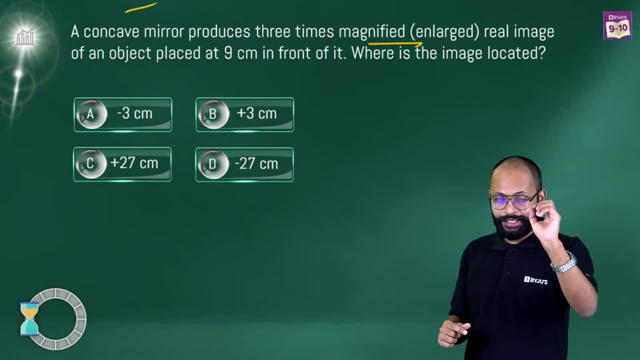 Right, So we'll have a poll question. I'll give you four options, And A, B, C, A, D. You can tell me which one is the correct answer? Right, Oh one. That's how it is. 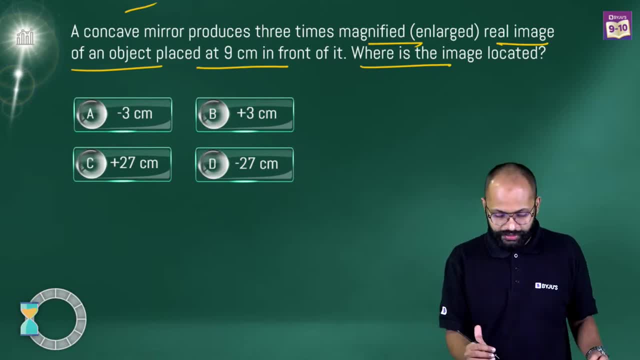 Right, Because that's the possibility. Cases are what? The possibilities? Where is the image located? So I'll give you 30 seconds. Try and answer. It's not that difficult. Come on. Your time starts now, So you'll get the poll in the chat itself. 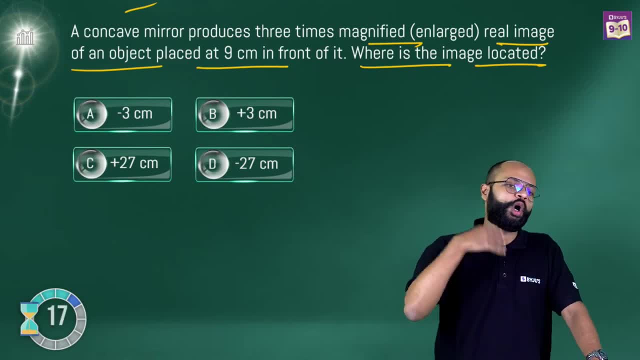 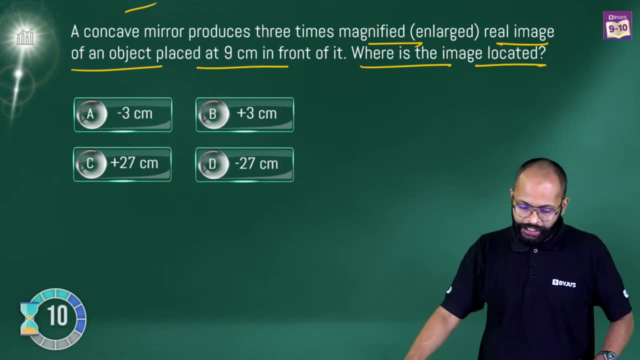 You can click on it. Which option do you think is correct? And I'll get to know how many people answered what option Right. So a concave mirror produces three times Magnified real image. Okay, Where is the image located? 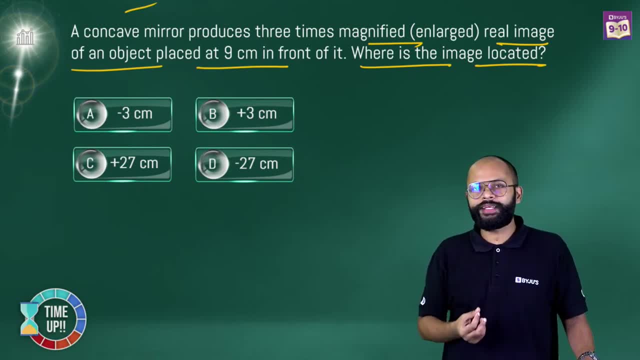 Focal length depends Focal and depends, If you, if you ask me what is focal length Where the all the rays converge, Right. So this is a value which you find experimentally, Right, Okay? So, Niu, that's the answer I'm giving you. 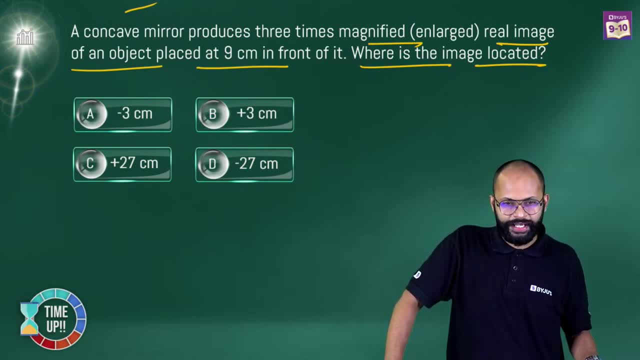 Okay, I can see minus 3 and plus 3 has a fight there, So how is it possible? Anyone with option D, Nice, Niu, I saw this. Yes, Rishi, Correct, 27.. D had 25%. 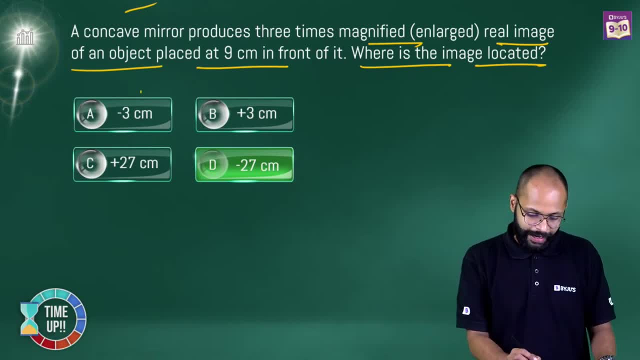 Okay, Maximum. people said option A, which means minus 3.. Why was it? Why was it? See, let me tell you something. When you, when you read this question, no, understand, there is something very important given to you. 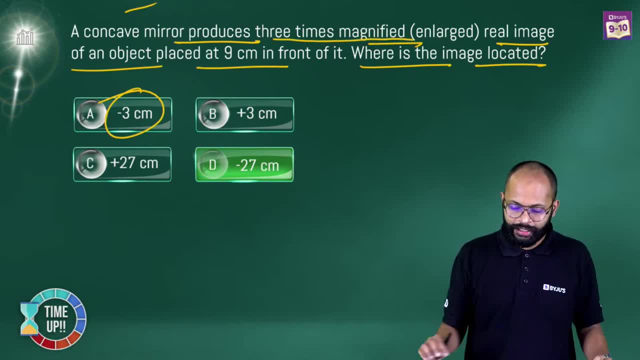 A concave mirror produces three times magnified real image. The moment the question told you it's a concave mirror, right, It is giving you a magnified image, and a real image Means means this is only possible. see a concave mirror magnified image and virtual is when it is between P and F, but it is erect also. that's why. 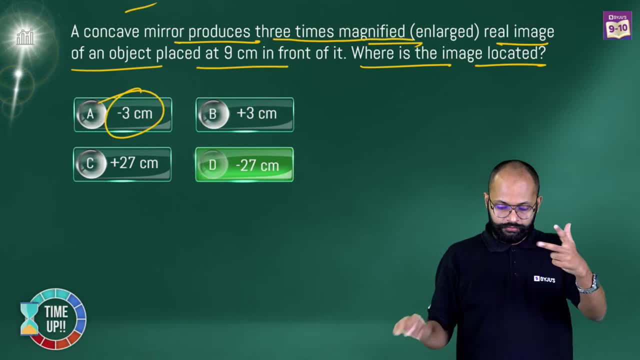 If it is inverted, right. if it is sorry. if it is saying three times and real- three times and real means it is, it is inverted also okay. It's okay, Shikha, It is inverted also right. 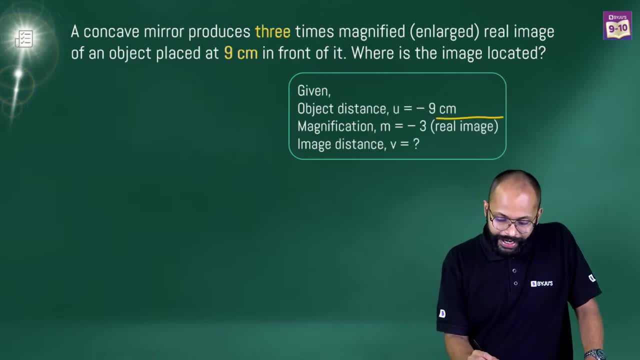 So that's why You will get to know. You will get to know that M is minus 3.. Who gave you this hint? The question gave you this hint. How, Telling that it's a real image? right, If I draw a concave mirror? this is focus and this is C. 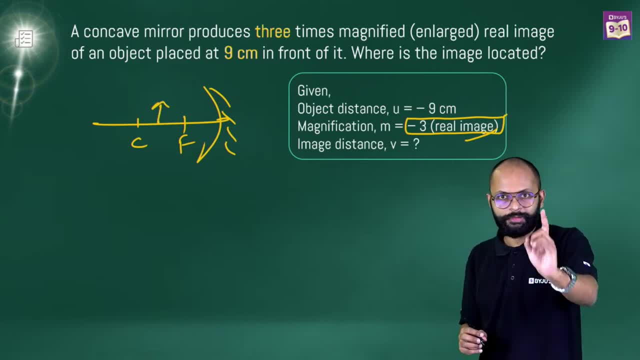 If I put my object between C and F? if I put my object between C and F, then only you will get a enlarged and real image right. Otherwise you will not get it correct Because real is given to you. So I am telling you these questions. 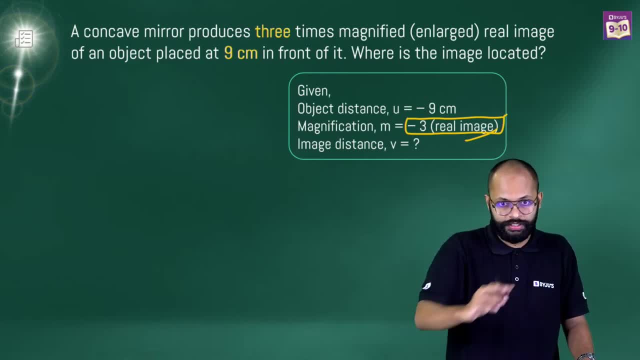 I will give you hints in such manners. Understand those hints. Very important, okay, Yes, No, no, Krishna, it is magnified and real Means it will be between C and F, right, That's why, Alright, So M is minus 3.. 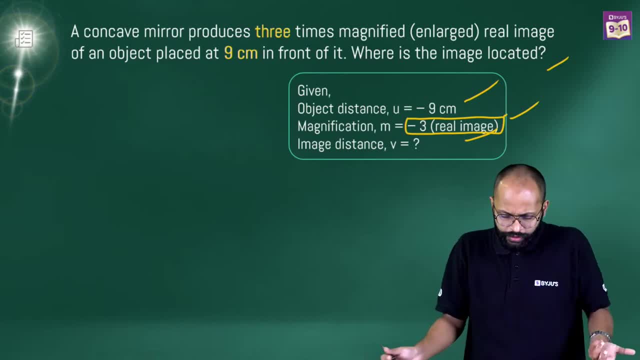 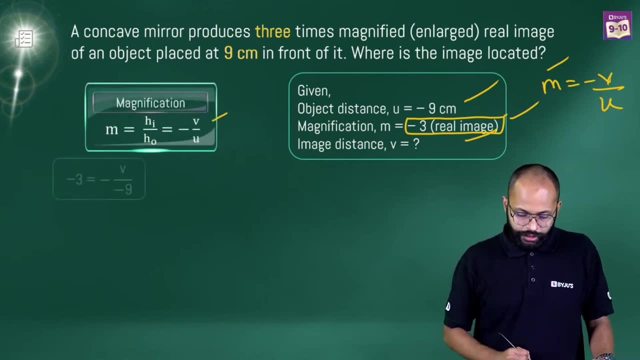 Object distance is minus 9 because placed in front of it you just have to find V. So you will use M equals minus V upon U, Simple right. So you will put use the formula minus 3 upon. 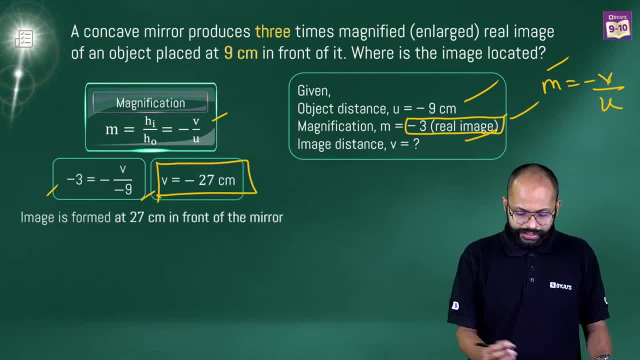 You will use this and then you will get what V equals minus 27.. Simple, Got it Somehow tricky And people. just one more thing: When you were saying minus 3, right, You were saying minus 3.. Understand. 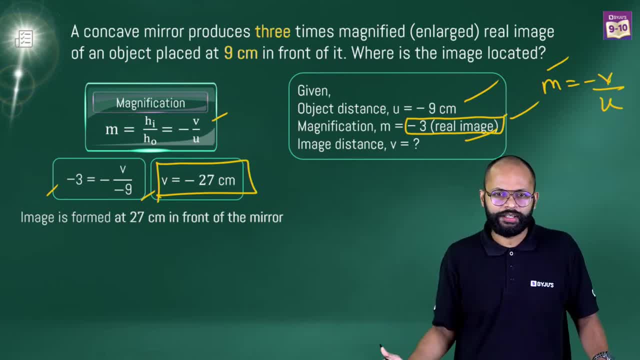 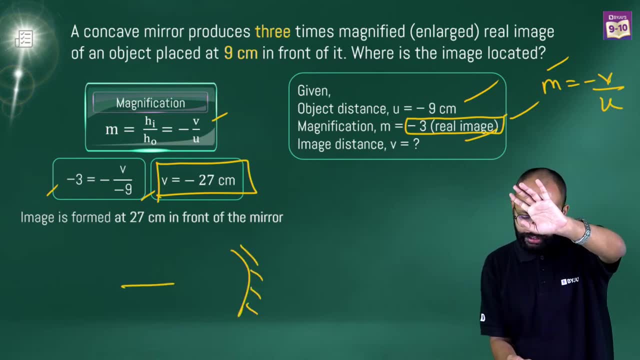 The answer you are giving. is it possible? Is it really possible? That object is 9 centimeters. So if you think, if you think the answer you were telling me, minus 3.. You are saying in a concave mirror object is kept like this behind, right? 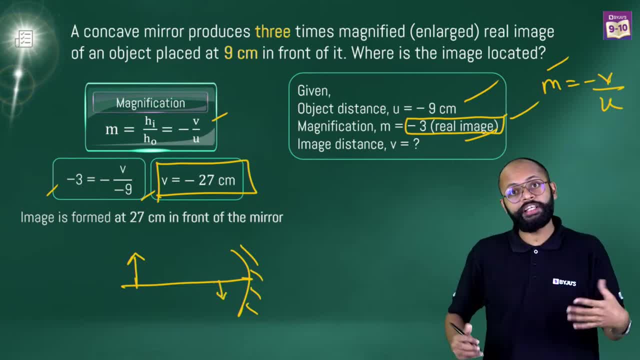 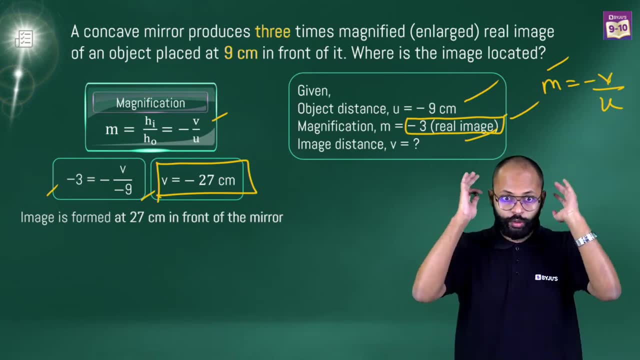 It is far from the mirror and image is near and it is enlarged. Not possible. No, This case does not exist. That's why I am saying: think You have to open your mind a little and do this. That's very important. 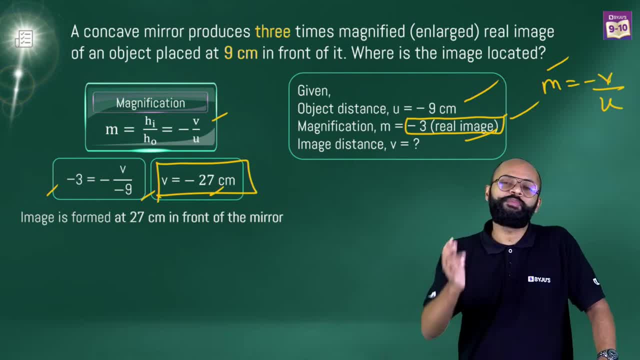 Yes, Right, So simple. V equals minus 27.. That's important And this will happen. no, If your object is between C and F means image will be beyond. It will be more than that. That's why. 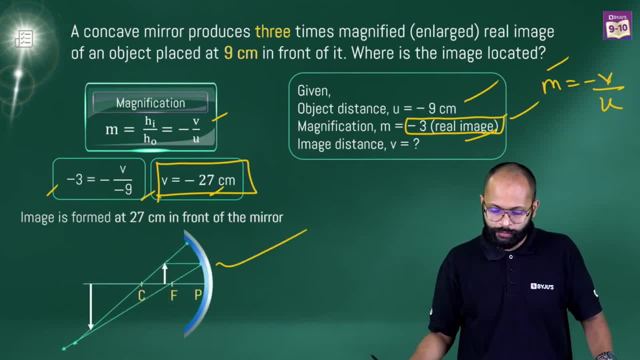 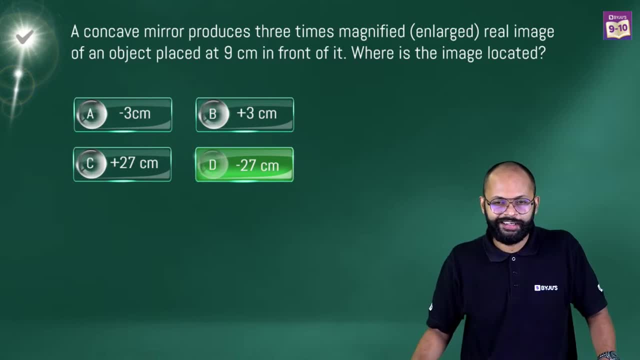 Correct, Super easy, Nice. So this is the case we are talking about, And that's why minus 27 was the correct answer. Okay, Understood, Right, We have few questions, Don't worry, Give me this question. 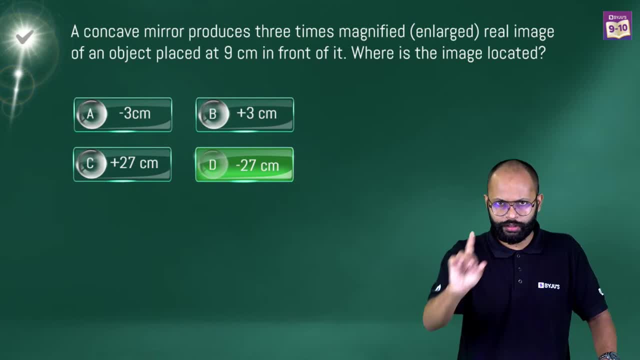 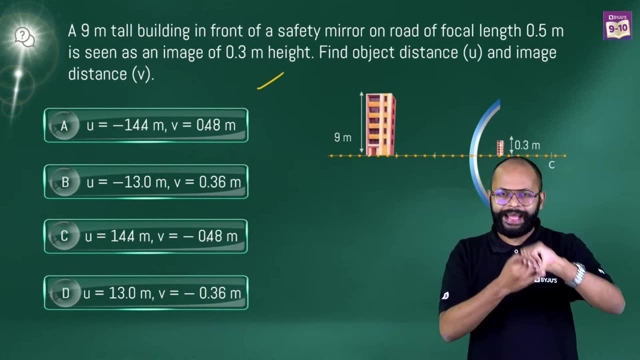 During the end of the session. I will have a look, But I saw the question. Yeah, I can solve it, Don't worry. Okay, Clearly understood, Very good, Very good, Very good. Next question. Next question A 9 meter. 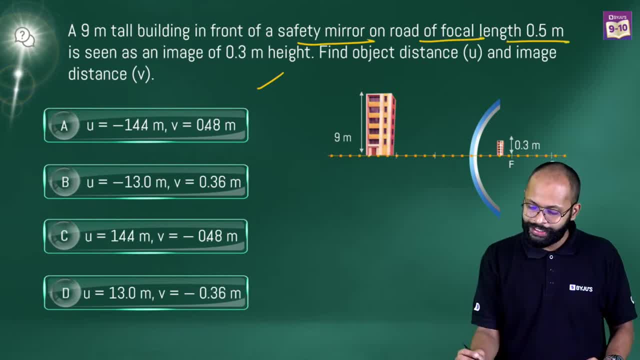 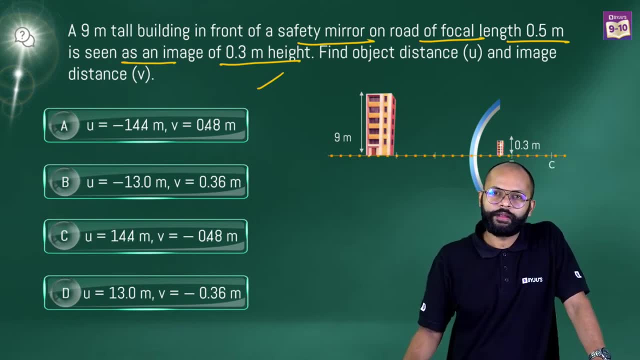 Tall building in front of a safety mirror on road of focal length 0.5 meters is seen as an image of 0.3 meters height. Okay, What is given to you? So, before seeing what you have to find, see what is given to you. 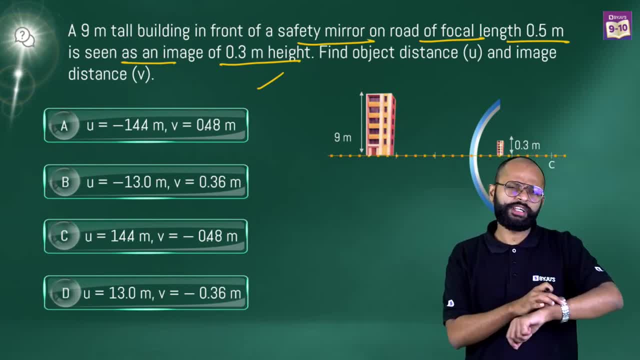 First of all, Right Abhilash, 15 minutes more Right. So a 9 meter tall building. What is given to you? Height of object is given to you, HO is given to you as 9 meters Above principal axis. 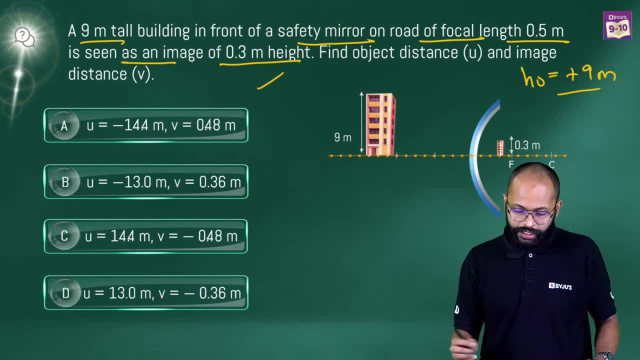 Means plus 9.. Okay, Nice, Plus 9 meters. Alright, Focal length is 0.5.. Now the question has not told you which mirror, But can you look at this particular keyword and tell me which mirror? 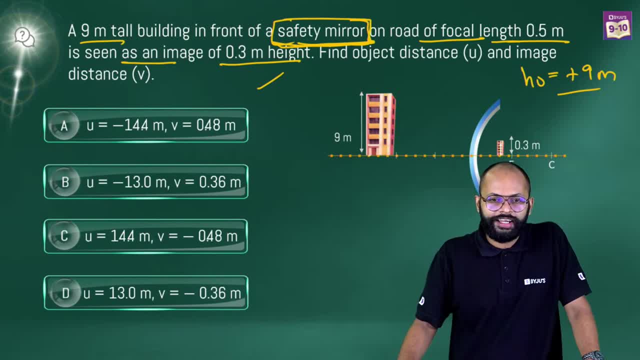 Right? Hey, Namesh, It's okay, I miss you. I miss you too, Right? So safety mirror. The moment you read this thing, you will get to understand: Oh, surveillance, Safety- Rear view Convex mirror. 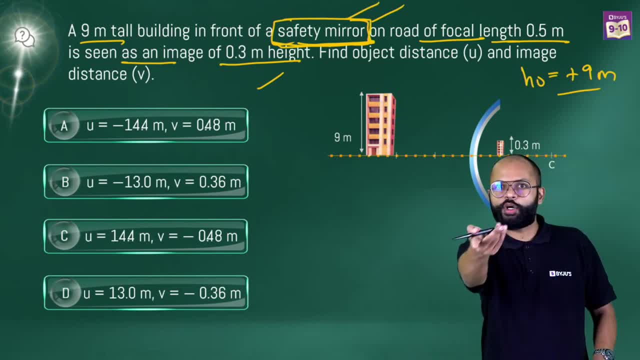 Convex Right. You will get to know just by seeing the safety mirror. It's a convex mirror. Okay, So convex mirrors focal length will be 0.5, which is given to you in the question. Okay, convex mirror's focal length. is it positive or negative? 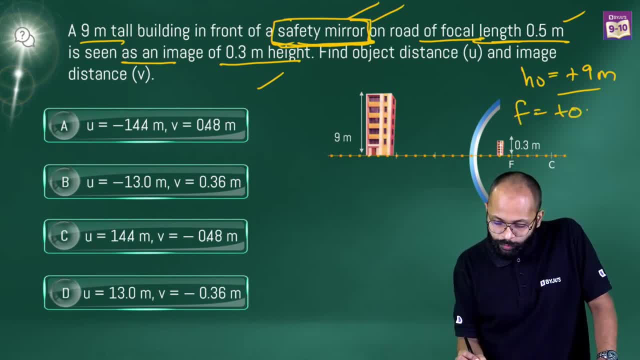 It's positive, No Right? So F is going to be plus 0.5 meters, Alright. Image of 0.3 meter height. Height of image is 0.3.. Plus or minus. Plus or minus. It's a convex mirror. 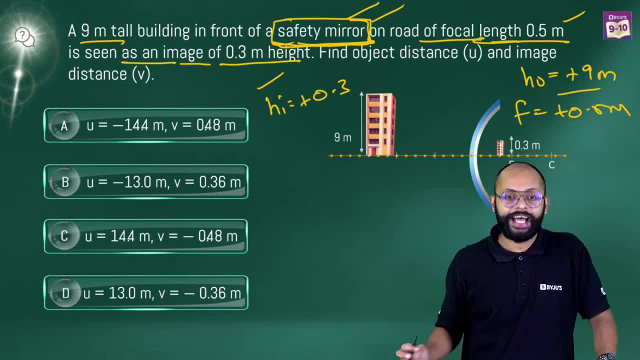 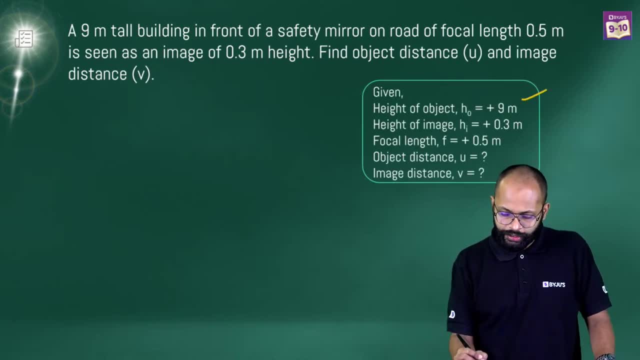 Virtual Erect Diminished Plus. That's why Nice, Very good answer, Right. So HI is plus 0.3. So if you have all these values, then you can use See. today my focus is to make you understand how to get to the mirror formula. 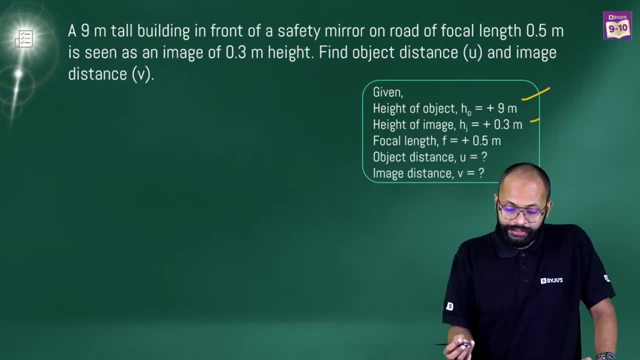 Okay, Calculations you will do, I understand, But understand this thing Very important: How to read a question, how to make sense of the question and how to extract information from the question. That is the most important step in all the numericals of flight. 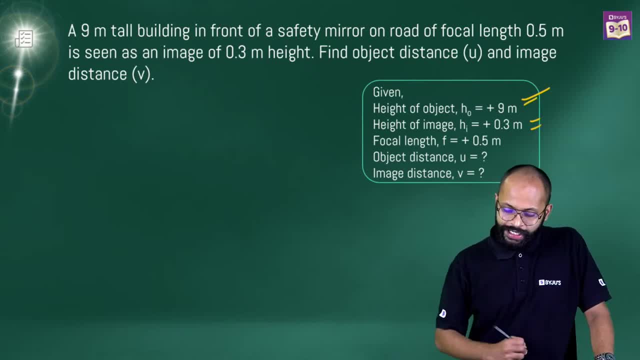 I'm telling you: Okay, So HO is plus 9,, HI is plus 3, and F is plus 0.5.. You have to find U and you have to find VA. Now, what to do Right Now what to do? 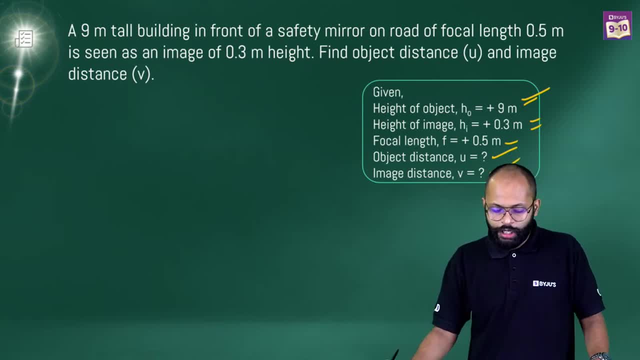 Okay, Everybody is saying B, Very good, Alright. So now what to do? Sir F HI HO, I have to find object distance also image distance also Means. you know what? I'll have to use both formulas. 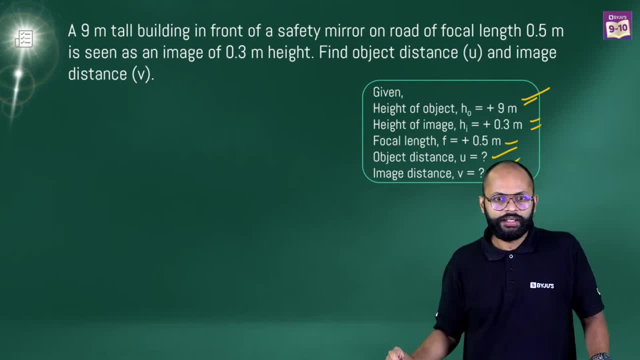 Magnification also and mirror also, Isn't it, Isn't it? It's okay, Rishi, Practice. Numericals need practice. The more and more you practice, the more and more use case you will see in front of you. The more you practice, the more you will see different types of numericals. 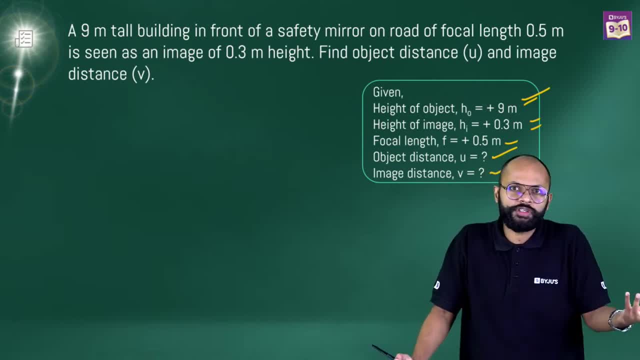 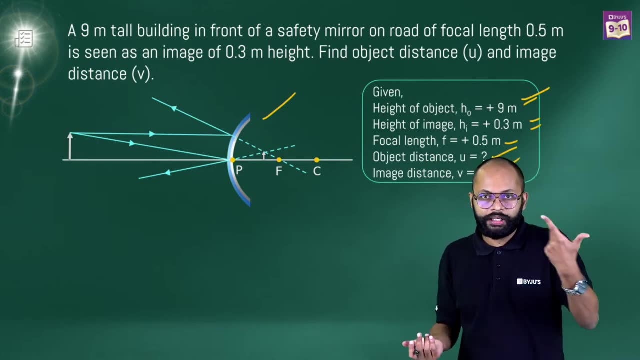 That many numericals you will see in front of you, And that's why you will become proficient. Simple, Isn't it? So, yes, Ray diagram, Because in convex it's always virtual, erect and diminished. Fine. Next, 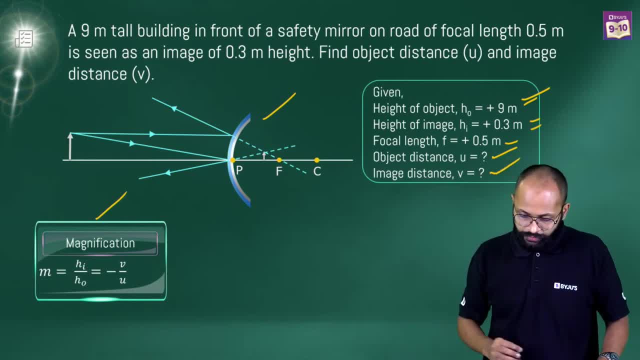 If you take into account the magnification formula- See when you take magnification- then what you will do, M will be how much M is given to you, as 0.5 equals Minus of V upon U. So can I say 0.5 is what? 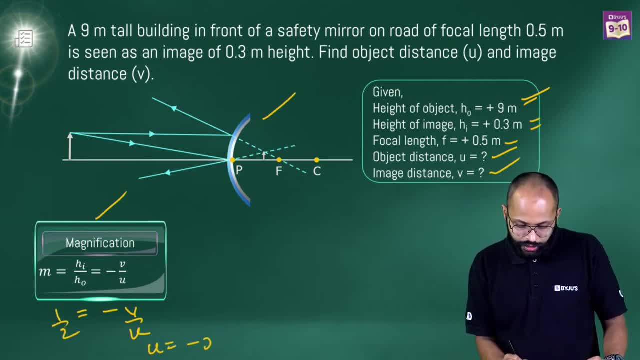 It is 1 by 2.. So I can say U is minus of 2V. So I have found U a relation between U and V. now, Isn't it, Ishika? I understand It will happen slowly, slowly. 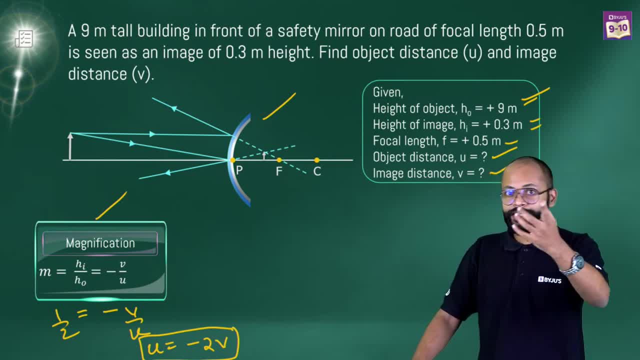 And good thing is you have time. The reason we are doing this today, The reason I am taking this session again, Or I would say extension of this session, Is because I want to make this understand to you very well: Kids get stuck here. 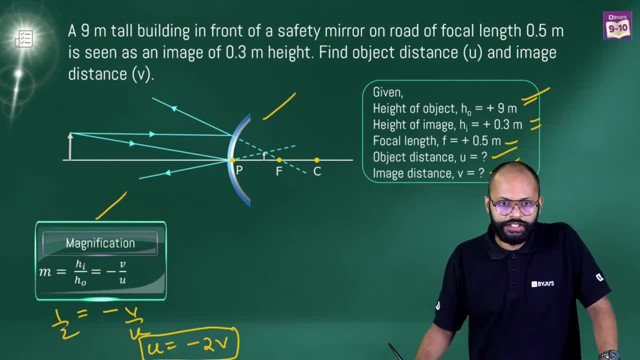 That's why I am telling you: Okay, It's okay, Taisha, Isn't it? So you will find relation between U and V. Fine, Now, if you got relation, You can use mirror formula, Because F is given to you. 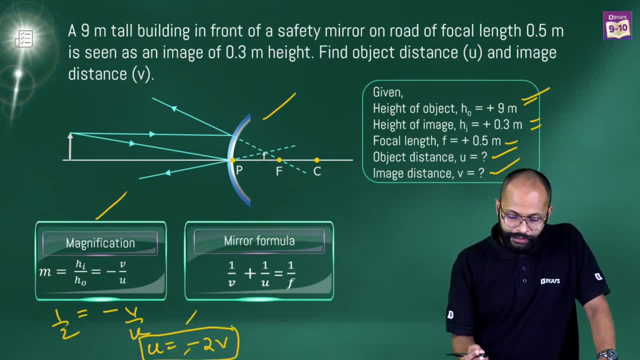 Right. If you use now mirror formula, You can put the value of U in terms of V And find V. If you found V, you will find U also, Isn't it Sir? how is M 1 by 2?? 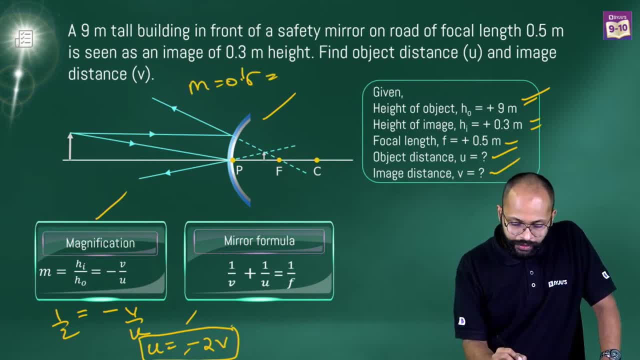 M is 0.5. 5.. You understand that. What is 0.5? 5 but a 10. Or 5 upon 10. It will be 1 by 2. Simple Right. That's why. 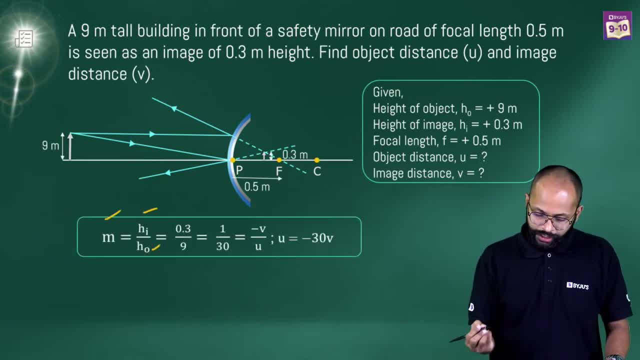 It's okay, Muskaan, Right, So now Let's solve it. So M will be HI upon HO Means 0.3 upon 9. Because height of image is 0.3. This is 9.. 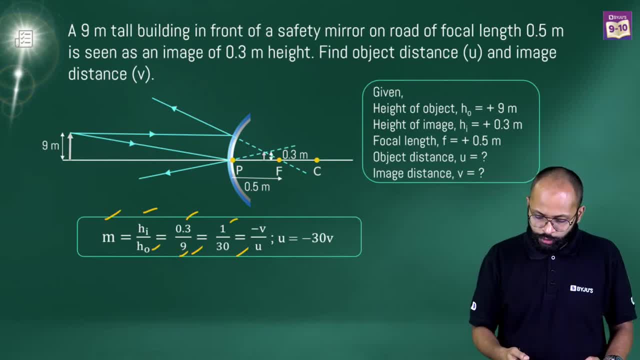 Means 1 by 30. And this will be equal to minus V upon U. And what you will get? U equals minus 30 V, Right Is it? Yeah? yeah, Sorry, Okay, Correct, Right, So it will be: 1 by 2 equals 0.3 upon 9. equals, yeah, equals minus V upon U. 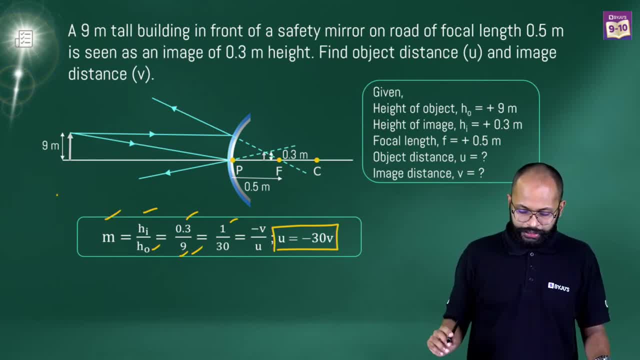 So it's simple: You will get minus 30 V, Right, Right. Oh sorry, I did one one, one mistake. This 0.5 was not magnification. My bad, My bad, Okay, Yes, 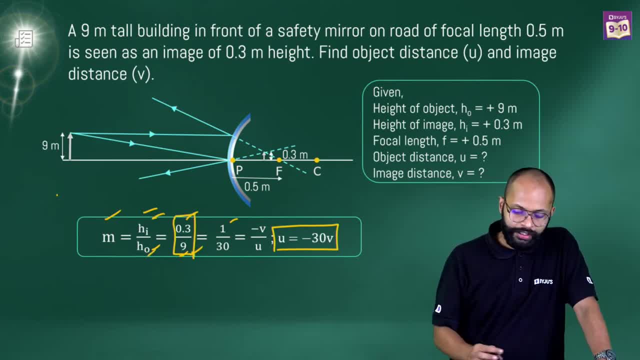 So M will be HI upon HO And this will be 0.3 upon 9.. So I took it as M. That's one mistake which I did. So this was F actually Right. Yeah, yeah, yeah. 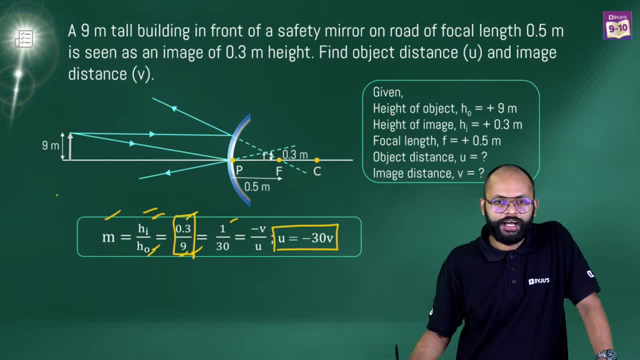 Neo, sorry, sorry Guys, I'm sorry, I did not see it. This is F, I just took it as M. It's okay. These kind of mistakes will happen. I'm telling you, The more and more questions you do, these kind of things happen. 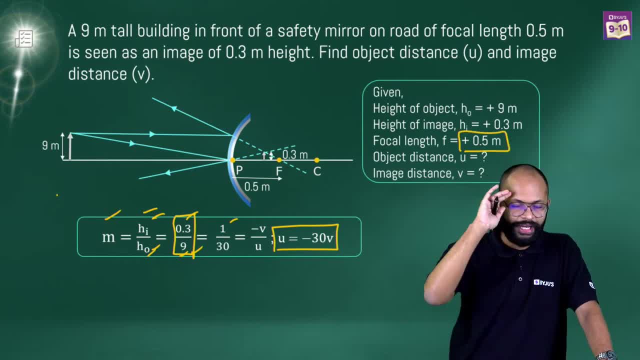 All right. So, yes, You will use formula of magnification First of all, height of image upon HO. Right, Yes, So M will be HI upon HO, And this will be 0.3 upon 9.. This is 1 upon 30.. 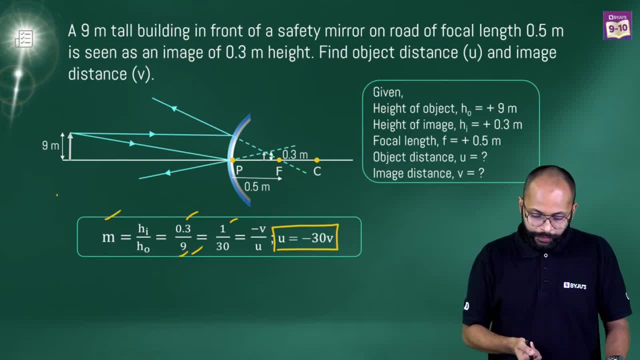 And then you will keep it equal to minus V upon U, And that's how you got the relation, as U equals minus 30V. Okay, Right, Yeah, It's okay, It's okay, Right. So you got both the relations. 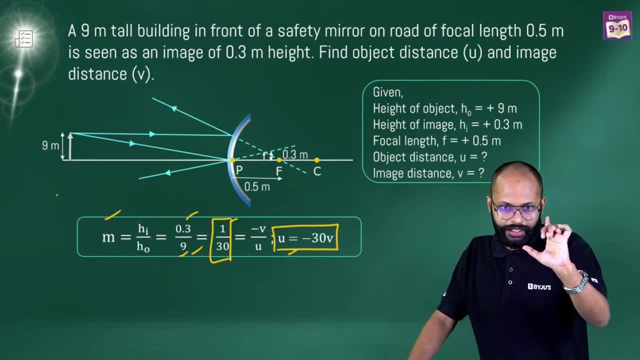 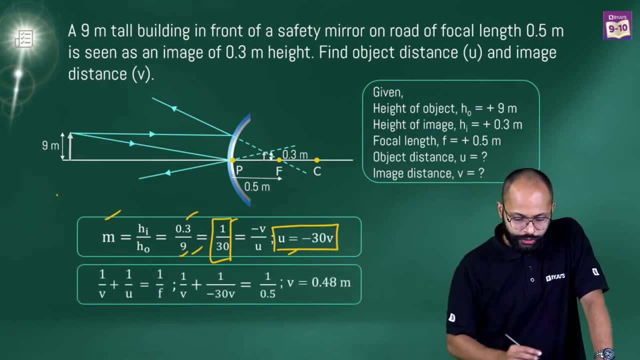 Now when you use it in this. So I kept the value of U as minus 30V, Okay, Yeah, yeah, It's okay, It's okay, Right, So you got both the relations Now when you use it in this. 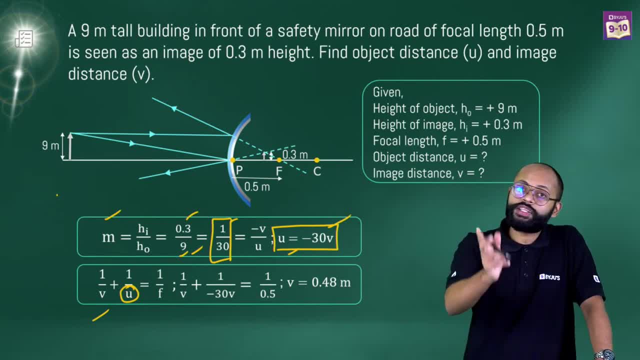 So I kept the value of U as minus 30V. Yeah, yeah, yeah, because that's what we found. So 1 upon V plus 1 upon minus 30V equals 1 upon 0.5, because F is plus 0.5. And when you solve this, you will get value of V as 0.48.. Right, Correct. 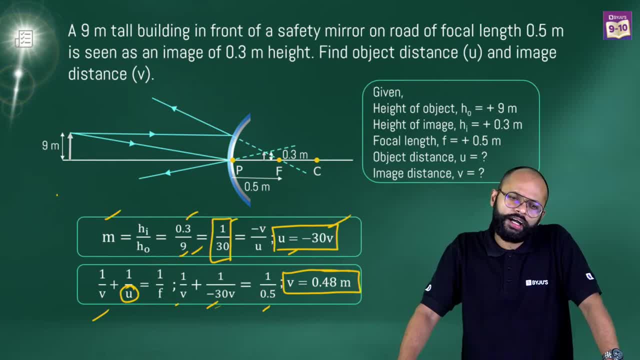 Yes, Krishna, Right. If you are saying to apply mirror formula first and then use magnification, I would say: hold on In magnification. you have two variables Right. So first you need relation between them. Who will give it to you? The magnification formula will give it. 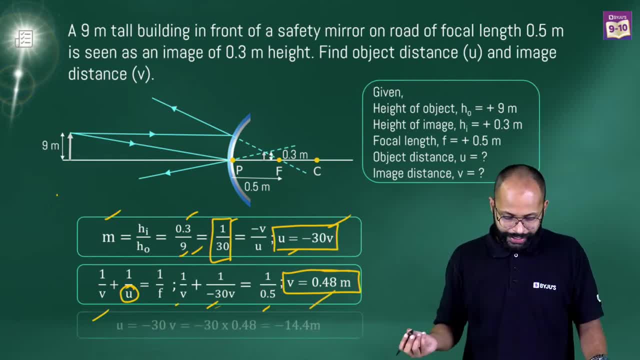 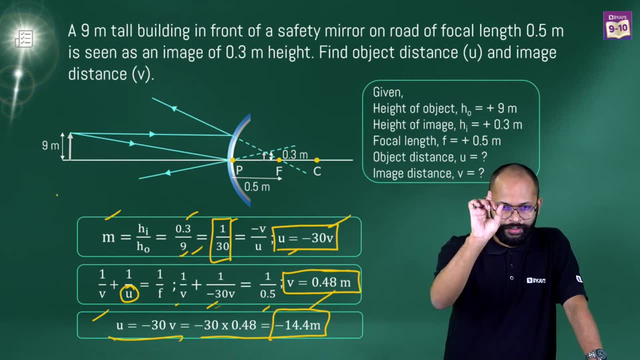 to you. Okay, Yes, So you got V and simple You can say: U equals minus 30V, You got minus 14.4. also Right, Right And just focus here. Mirror formula is confusing. I understand. 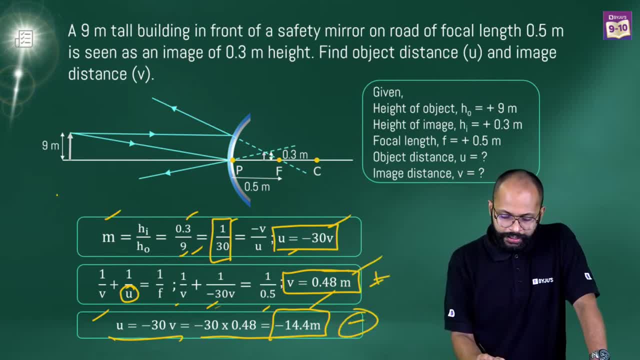 V you got positive and U you got negative. Your answer is correct, Sir. how do we know? It's a convex mirror. Means V is going to be virtual, erect and diminished, And on the other side means it is going to be positive and U will be negative. 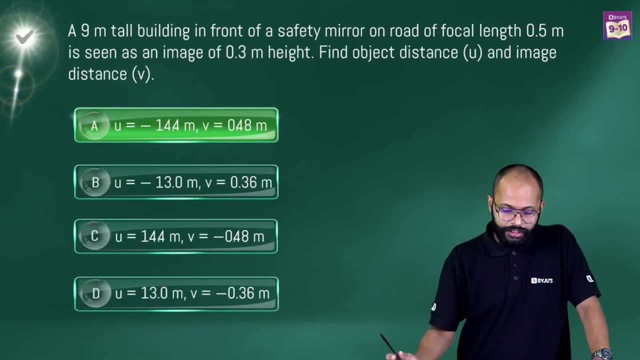 It is on the front side, Correct, Right. So and one more thing I just want to focus: See, in MCQs, don't waste time in solving it completely. If, let's say, tomorrow this question comes in exam, what I would suggest is, the moment you found 0.48, check all the options. If 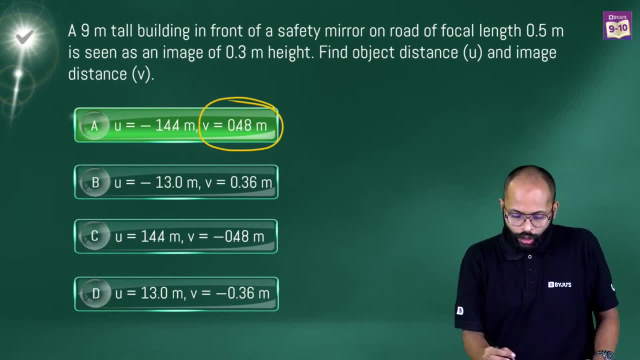 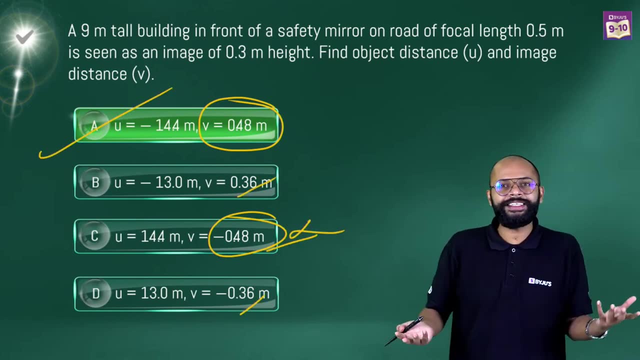 you have this As a unique option, Now 0.48. if you got it is somewhere else, This is minus, Which means not correct. 0.36, 0.36 means very easily. you can straight away say option A is correct. 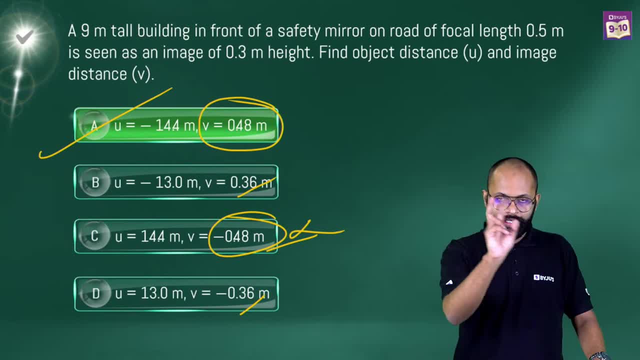 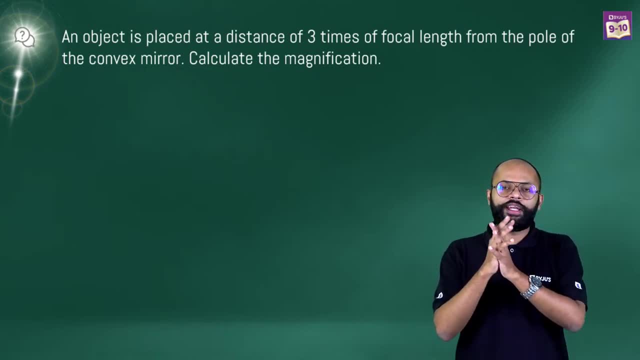 Why do you need elimination? Correct answer, Right. So that's why, In such kind of a questions, you have to play smart, Do it Fine, Eliminate options- Okay, Next question. next question: An object: Focus Right, Getting it. At least it will be happening, If you understand at. 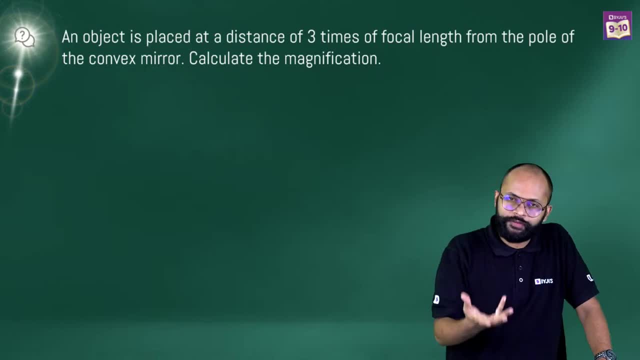 least 30-40%. If your confidence boosts, then it will be good. If you understand it. it will be good If your confidence boosts up 30-40%. also, you know what it's a success, Because I understand you need practice in this And you know what we'll do: a lot of practice. 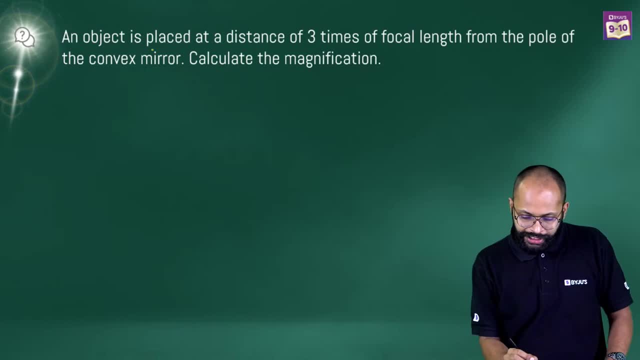 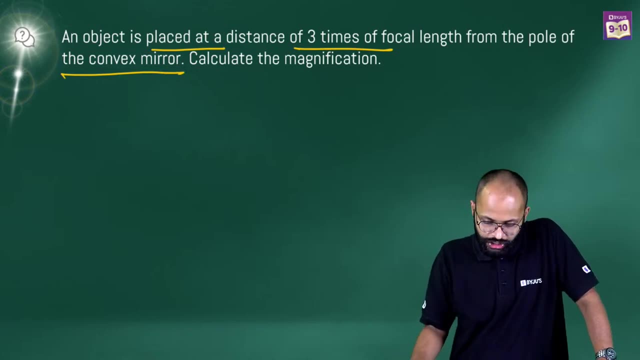 But today absorb it slowly. Right, An object is placed at a distance of 3 times of focal length from the pole of the convex mirror. Calculate the magnification. Now tell me What is given to you. Object is placed 3 times of focal length from the pole of convex mirror. 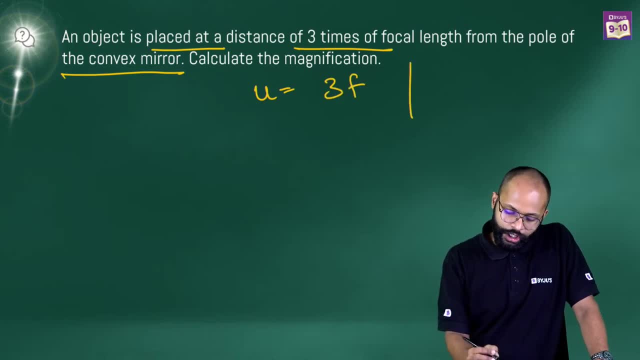 U is given to you as 3 times of F, Alright, And let's say the focal length is F, Alright, Alright, Now calculate the magnification. Yes, And your focal length will be positive for a convex mirror, Right. So F is going to be plus F. Why, sir? It is a convex mirror. 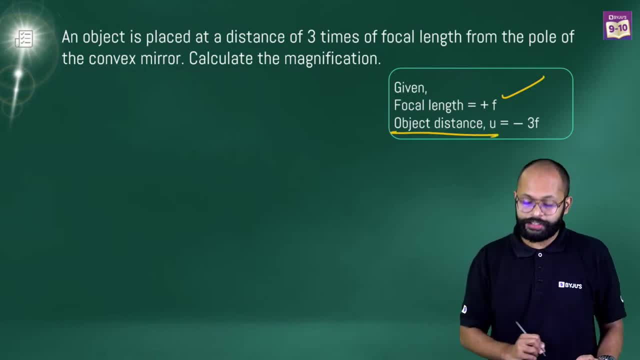 F will be to the right Means. it will be plus Correct. Object distance U will be minus. Sir, how do we know? U is given to you as 3 times of F? Alright, And let's say the focal length is F, Alright. 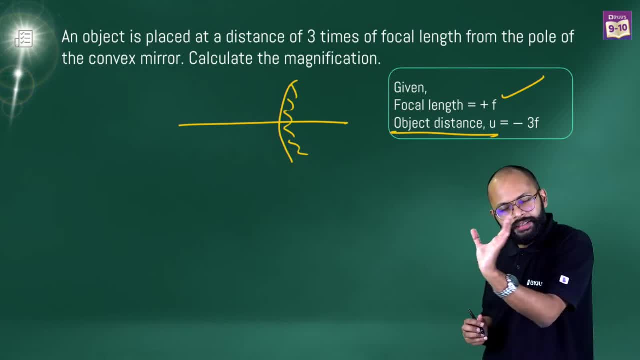 that's why I'm saying always have a rough diagram in the rough work area. F is going to be positive. it's a convex mirror. okay, sir, now you will be to the left. no means you is three times of focal length. means 3f surplus or minus. 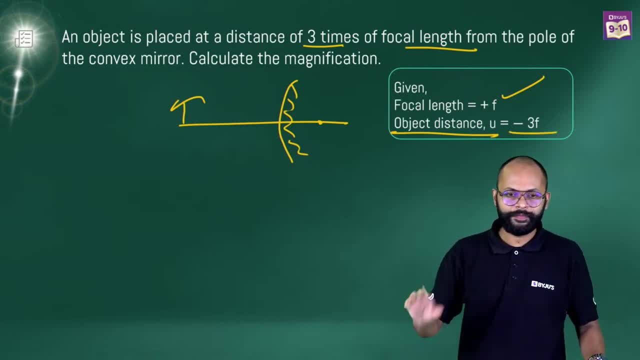 minus white because to the left. that's why you becomes minus 3r. simple, got it right. and uh, nice, if you got this much, apply mirror formula. you have F, you have you, you can find V also. and uh, it's okay, Rishi, the reason I'm saying this is: 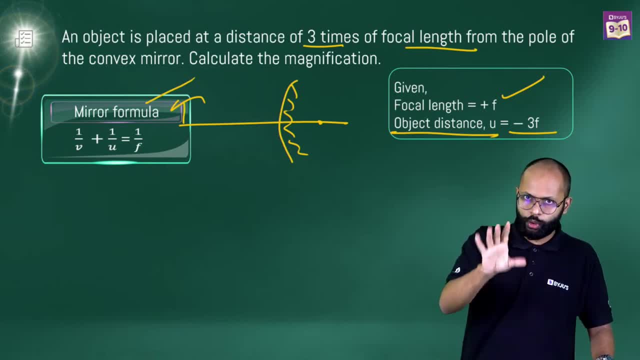 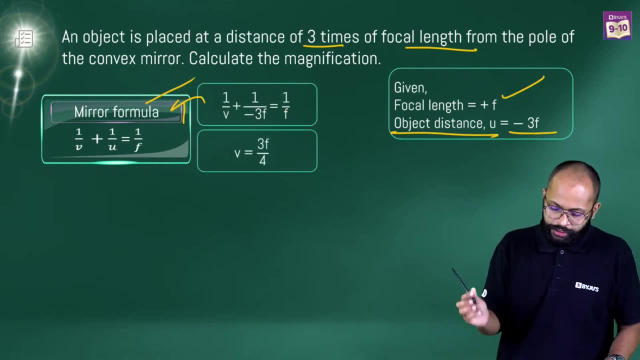 okay, it's okay. if you watch the session again, at least all these questions, do it, and don't worry, we'll give the notes to you in the telegram channel also, so you will have all the questions. so when you apply the mirror formula, you will see 1 upon V and same things, and when you solve, V is plus, which is okay because 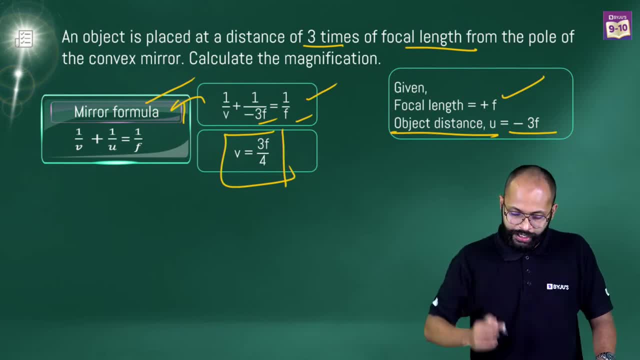 it's a convex mirror, it will be plus, it will be to the right. that's why so we came out with 3f upon 4, so we came out with 3f upon 4, so we came out with 3f upon 4. 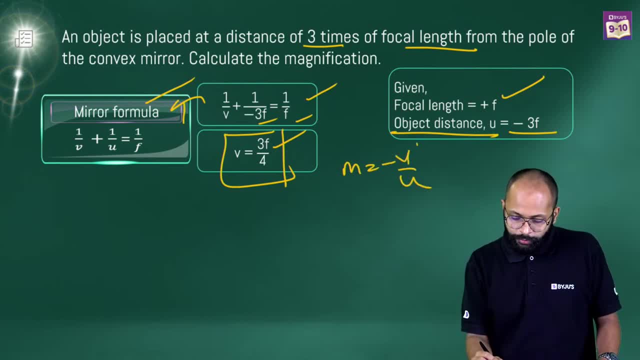 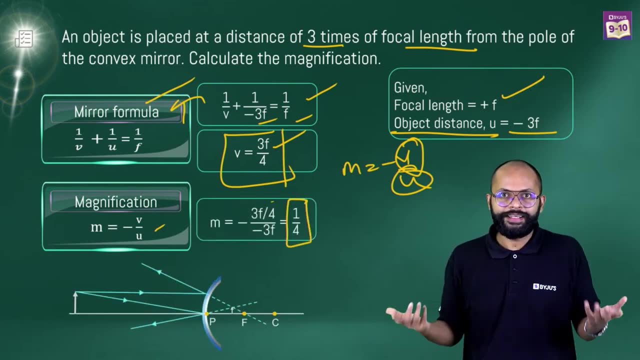 now, M equals minus V upon you. put the values of U and B right, put the values of U and V, you will get 1 upon 4. yes, it's supposed to be less than 1 because it is diminished. true, Anna neo, 1 upon a. hacha, tika, hacha. you have given the 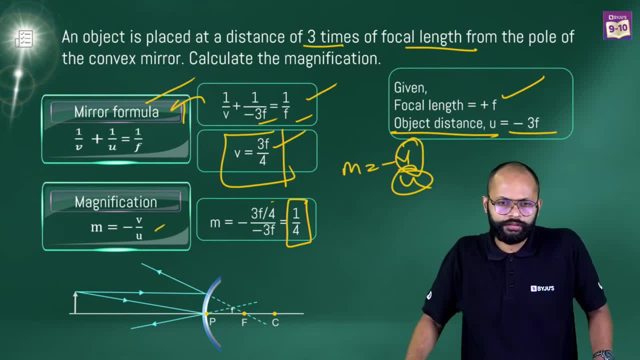 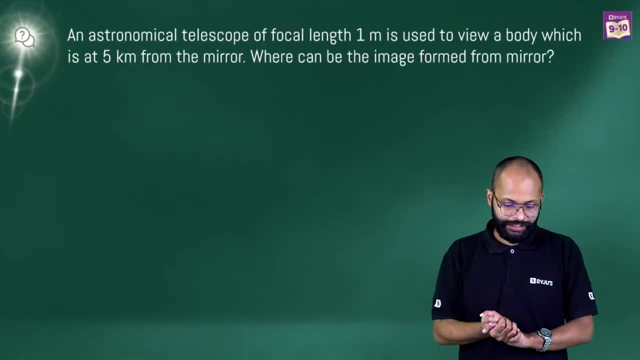 sword equation, I mean at least the restructured equation. that's okay, right, nice that we she very good 1 by 4, all right. so I said, oh, this question it is also a good question. the reason I'm saying it's a good question is because 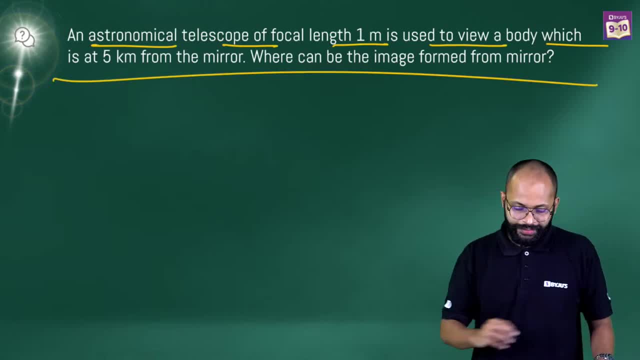 of one reason I'll tell you. an astronomical telescope of focal length 1 meter is used to view a body which is 5 kilometer from the mirror. nice, most kind of thing. got it, and in last session, I remember, and you were struggling now, good, all right. where can be the image formed from the mirror? which better is? 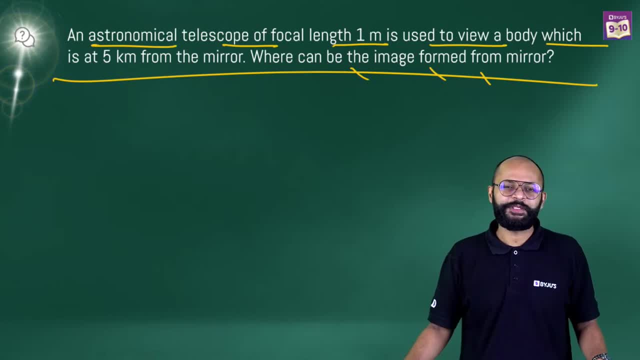 this anyone? which mirror is this? any idea? ha, f is one that's okay. focal length is one good, good new. can someone to say, ha, it's, it's ok. neither it's ok, it's a concave mirror. it's a concave mirror. see, I understand this is not exactly we have taught you till now, but still I'm giving. 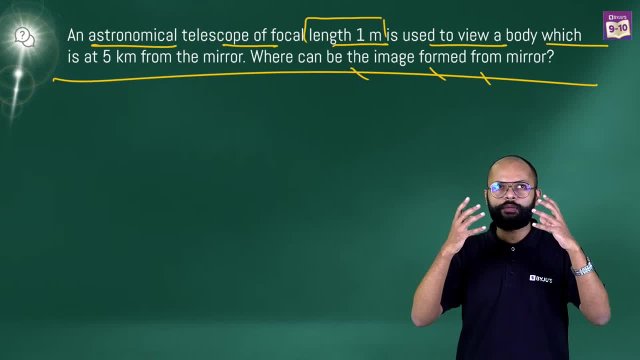 you a small idea: astronomical telescope. why do we use this telescope? first of all thing it is: you start to see very far objects means I can say almost infinite, and you can say almost infinite very far that telescope, astronomical objects, moon, star, Sun, all these things are not ok. now you want to see very far objects and you 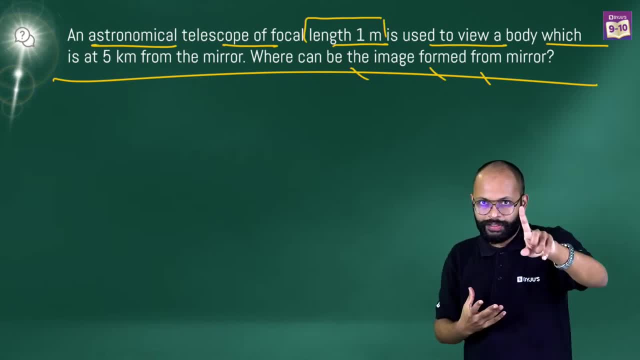 want to magnify their image also correct, that's one thing. but you know what, in these astronomical telescope, this concave mirror segment is half story. after this we magnify. so I'm telling you, first job is to focus the image. that's important to see long. 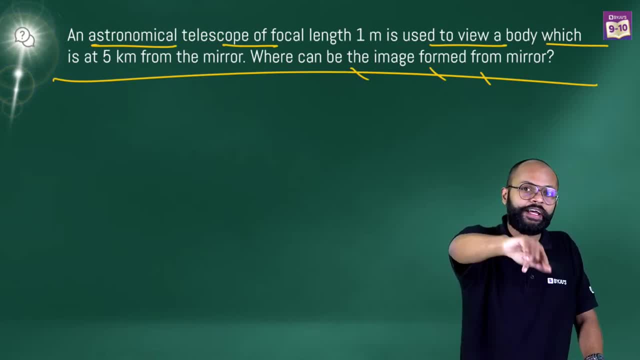 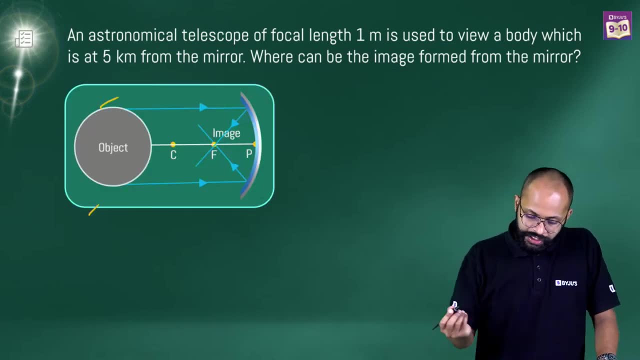 distances. the first job is focus, next job is a magnify. so this question asking about the first thing, the focus part, are nice. so how to do it? object which is very far from you. first of all you need to focus it, make a sharp small image and then you magnify. 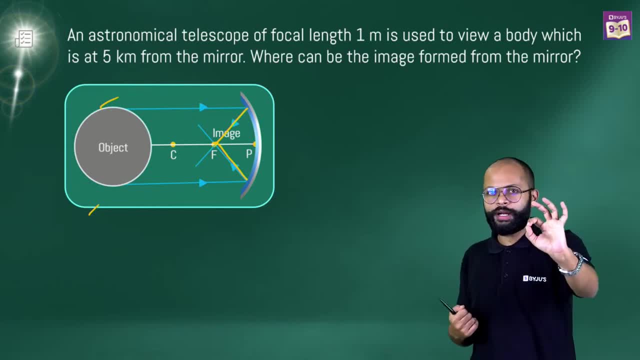 it don't worry, we'll study this in further sessions, but today I'm telling you the half story, and this is like probably part 1. understand it? so this is the half story. you have to focus the image, and that's where the concave mirror is. 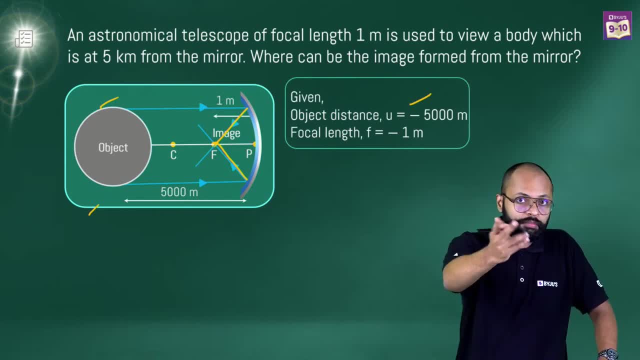 coming into picture. right, you equals minus 5,000 meters because it's given five kilometers. ok, right, f is minus 1y, minus 1 because you just told me it's a concave mirror and concave mirror has negative. that's why, and beyond center of curvature, yes, or? 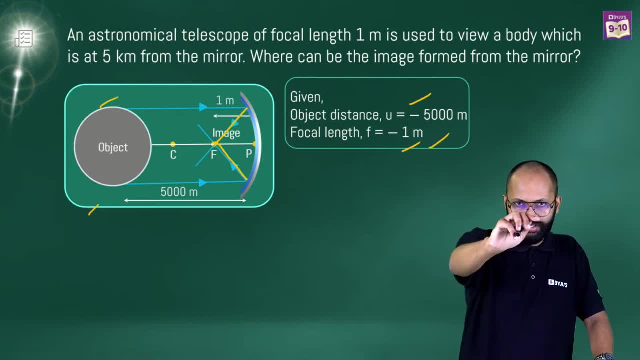 you can say infinity and you know what Anshul. actually, your answer is better than mine. the reason is because we'll solve it and understand what's coming when you use mirror formula. question is where the image will be formed. so 1 upon v plus 1. 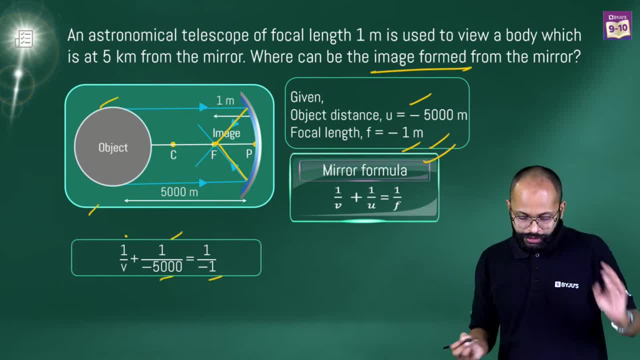 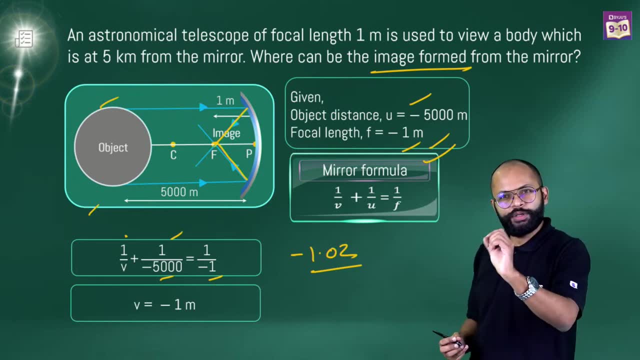 upon u. right equals 1 upon f. when you put the values and when you solve it, you will get about minus 1.02, minus 1.02 images at the focus. so I think someone asked me this question in the in the second-last was. 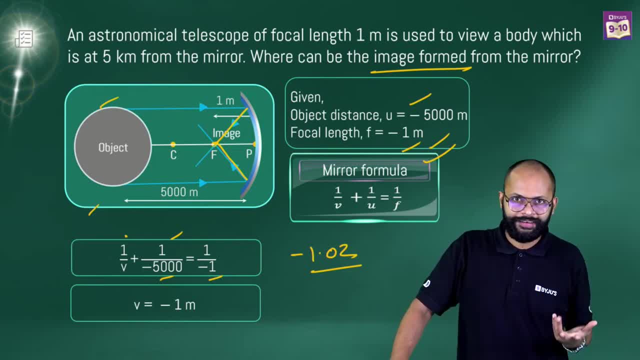 last two, last sessions, the third, last session. so how far? you won't never. you will never know how far, but you will know it when you solve it. so five kilometers, I told you intuitively. what do we? it's very far, it's like infinite answer is telling you: if you are getting minus 1.02 and focus is minus 1, it's at. 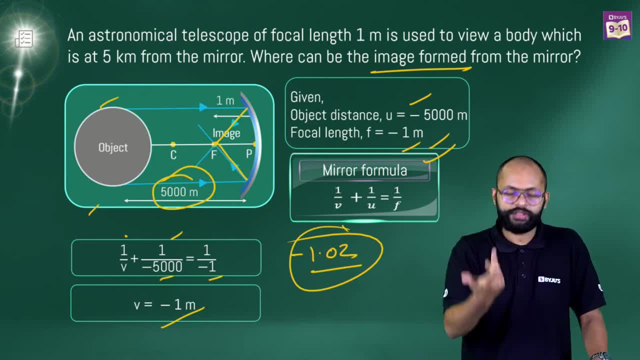 the focus only right, right, okay, got it. so that's why v is minus 1. it's at the focus means object. right, okay, got it. so that's why v is minus 1. it's at the focus means object was like infinity. Correct, Ishika, it won't be. There is a slight calculation mistake. 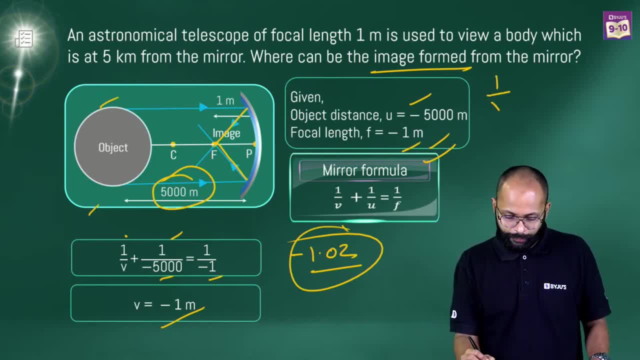 It won't be The reason I'll tell you. it will be: 1 upon V equals 1 upon 5000 minus 1.. It won't be 0.. Image is at focus at same side, Correct? So that's why? Okay, let's. 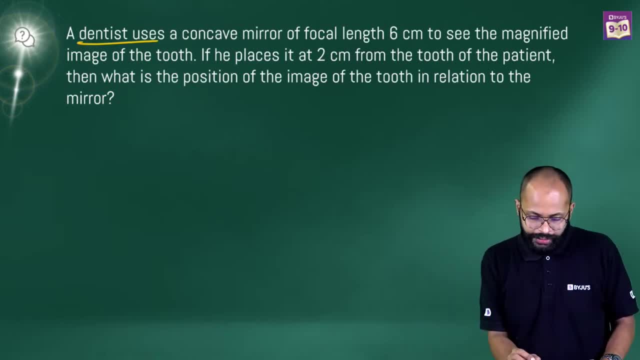 do this very quickly. the last question: Nice, nice. I need your help, guys, I need your help. Dentist uses concave mirror of focal length 6 cm to see magnified image of the tooth. What is given to you? A concave mirror, Okay. concave means f is going to be negative, Alright. 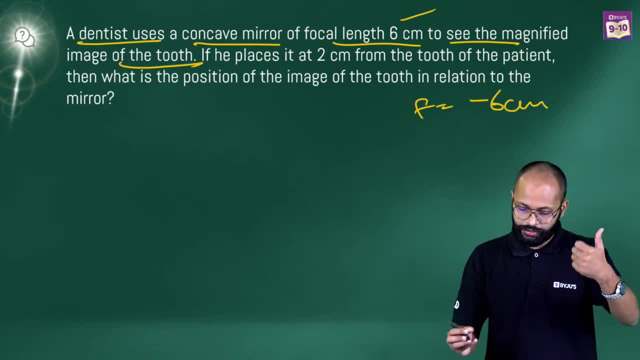 Focal length is minus 6.. So f is going to be minus 6 cm, Alright. Magnified image of the tooth. Sir, magnified image of the tooth means object will be between pole and focus. This we know. Nice Tabeshi, Correct Right. Yes, If he places 2 cm from the tooth of the 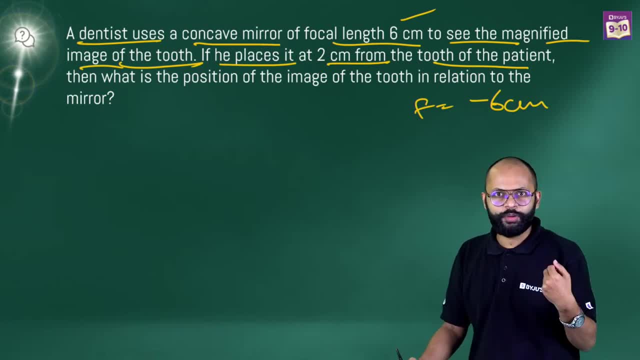 patient. that's what we said, Right, That's what we just told to our mind. Okay. object will be between pole and focus. If f is minus 6, u is given to you as minus 2.. Question even is: telling you 2 cm from the tooth, Then what is the position of the image of the tooth? 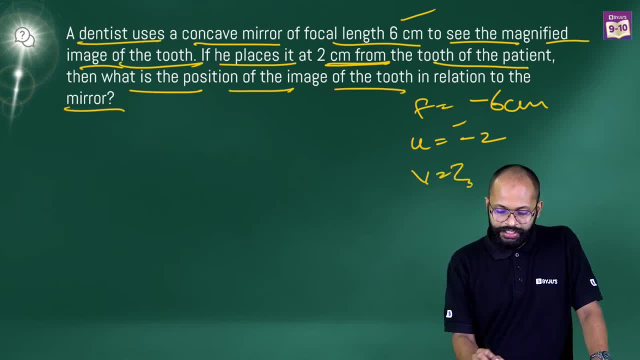 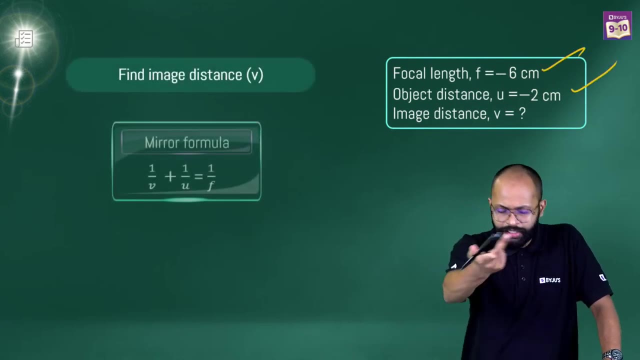 in relation to the mirror. What is asked? V is asked. Is it a difficult question? No, Simple question. Language looks big. It's a simple. it's a simple, easy question. No, Right, F is minus 6. U is minus 2.. V is something which is asked, Simple. Apply the mirror. 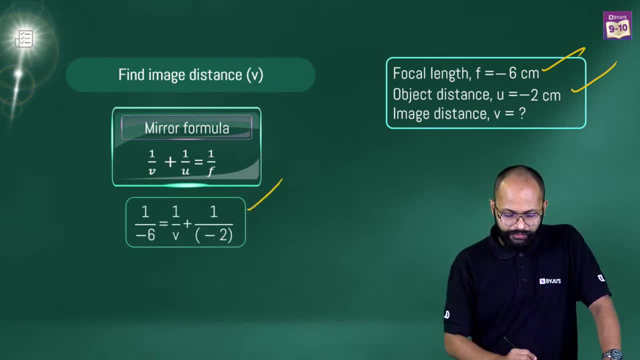 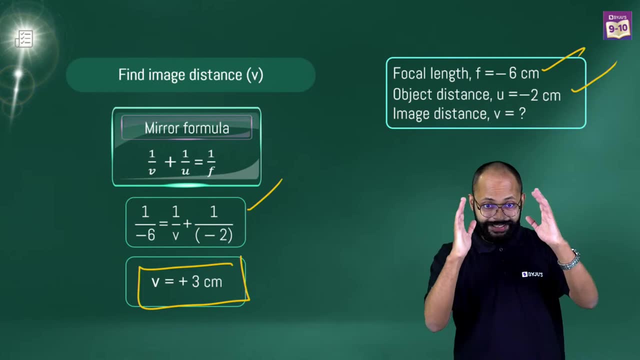 formula, Enlarge the image Right, Easy. So you can find V and you will find that plus 3 cm Right. Got it Easy, Right. So in today's session I am letting you know that don't be scared of mirror formula and magnification, Don't worry, We will do multiple questions. 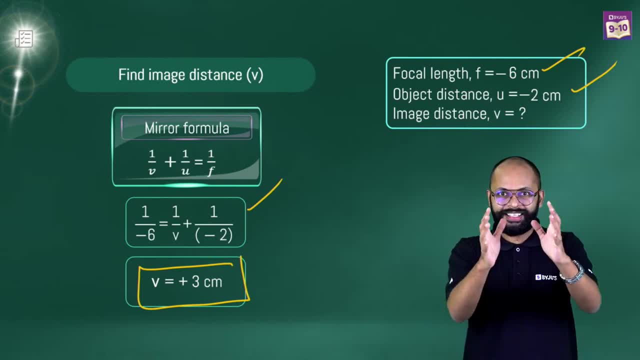 high level questions, But today's session was to get this fear out of you. Don't worry, We will do multiple questions, But today's session was to get this fear out of you. Perform step by step. Yes, it's new. Okay. Step by step. See what is there in Maths. 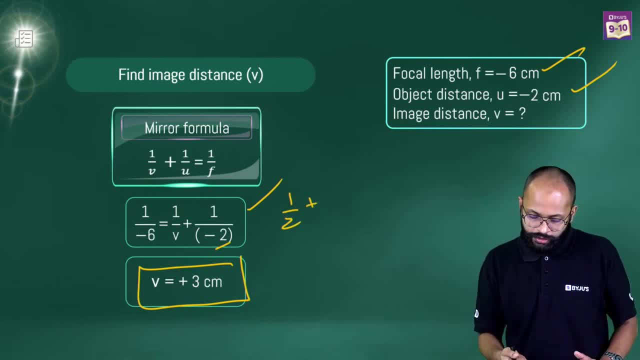 In calculation. I don't want to waste time, I can use it. 1 upon 2 minus 1 upon 6 is equal to 1 upon V. 6 will come 3 minus 1. So 2 upon 6. You get 6 by 2.. You get 3. Simple. 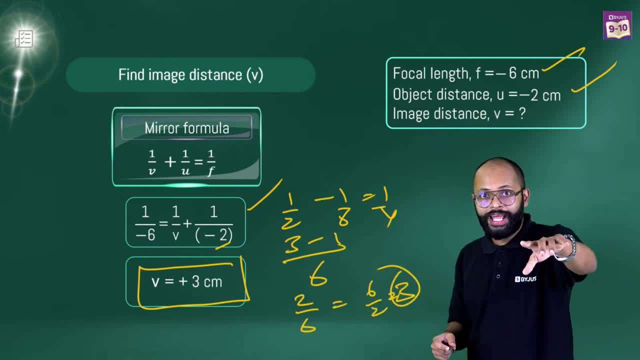 Right In calculation. I am not wasting time because your time is more important than this calculation, Right? So I am sure we will do it. We will do it Right. That's why It's important thing is to get the concept right, Because if that comes calculation, the more 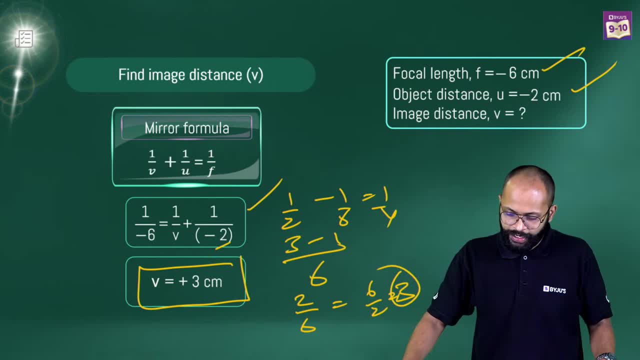 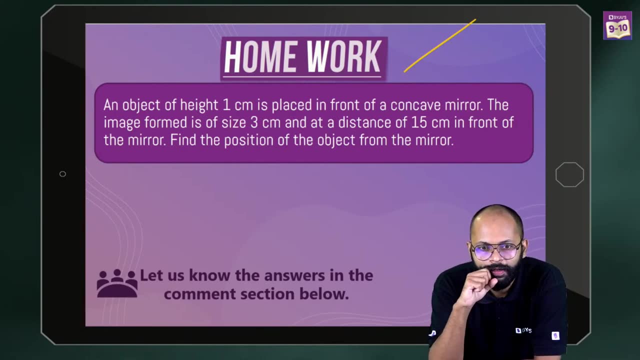 numericals. you do, you will get it Right. It's okay Easy, Fine, Today's homework question for you guys. Yes, Take the screenshot And I want to see answers. Right, I want to see answers. Okay, it's not Why I am taking reciprocal. Okay, So son, 2 by 6. You got? 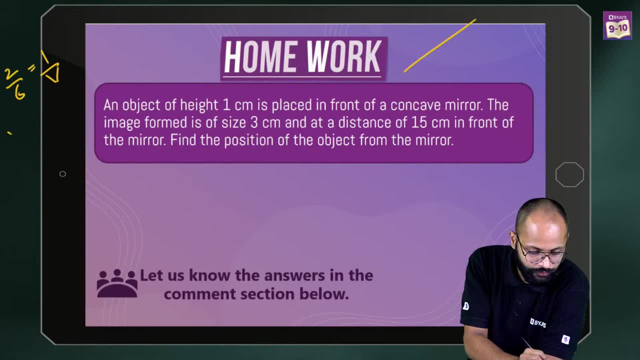 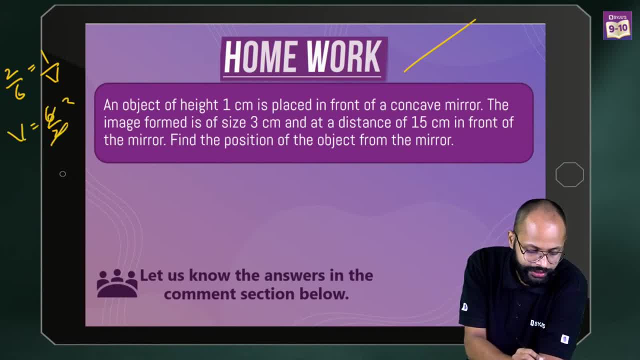 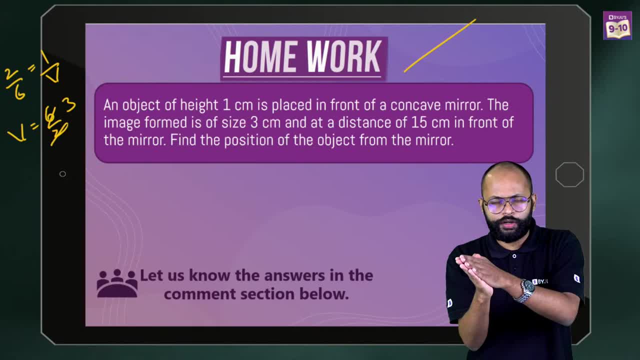 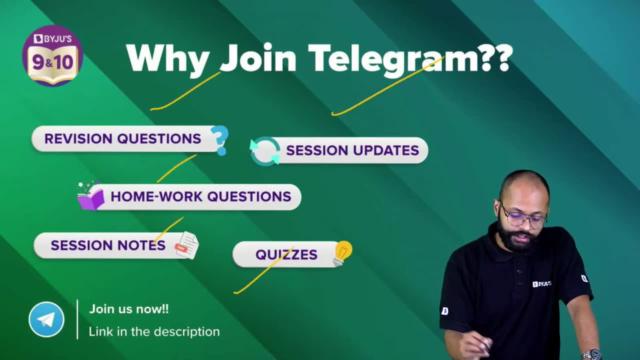 a lot of numericals together, Don't worry about this. So, homework question. you have seen, Telegram channel is very important. Okay, Yes, Bulb in a torch light, Okay, Torch light. may at least you know It's a concave mirror. Right, You have U. Right Now the 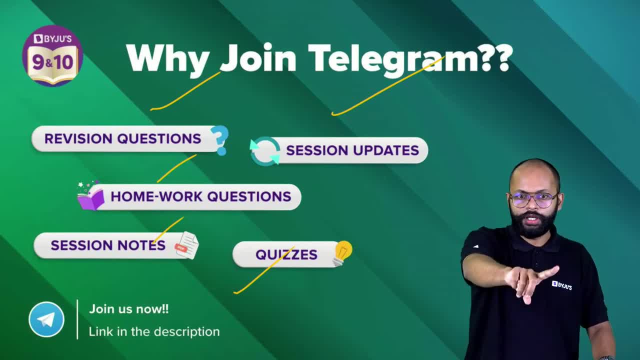 right, you have you. right, right, you have you. the question might have also given you the focal length. take it and you know what. one more thing you can see. if it's a torch light, you can take a case that you will be at the focus and we 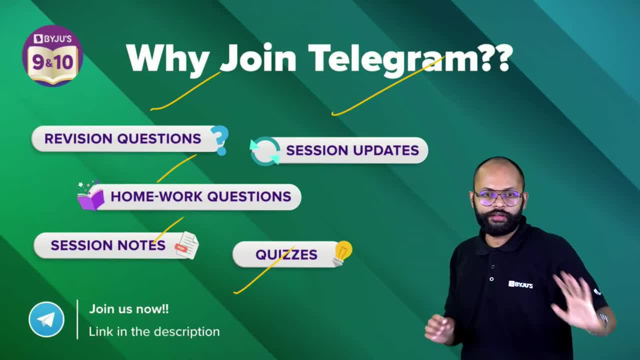 will be infinite, right into the concave mirror. got it? take a new answer. the question: torch concave mirror object will be at the focus. image will be infinite. you can take it finite. that's it. so telegram channel guys, join it. you will get the questions answer solution notes in that. so please make sure that. 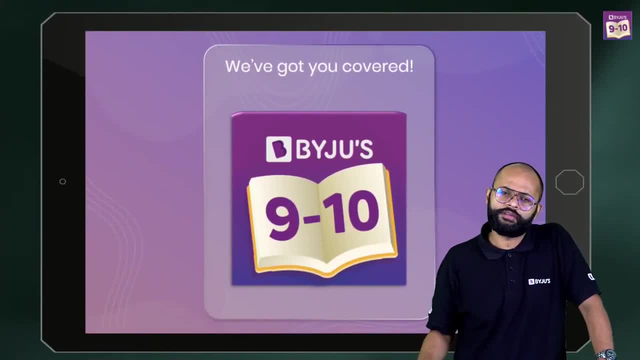 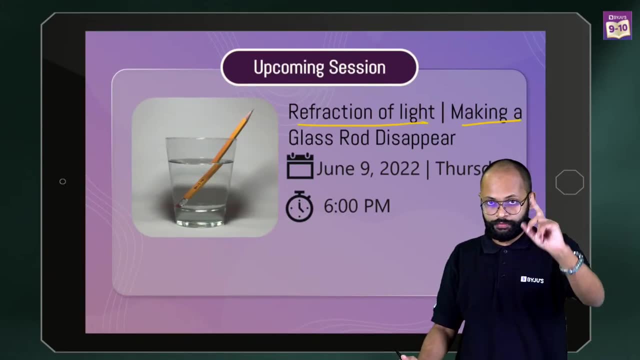 you are a part of this. and, last but not the least, we have got you covered. we tell this to you every time. alright, next session will have on refraction of light. by the way, today I was supposed to take this session, but because of you guys, I 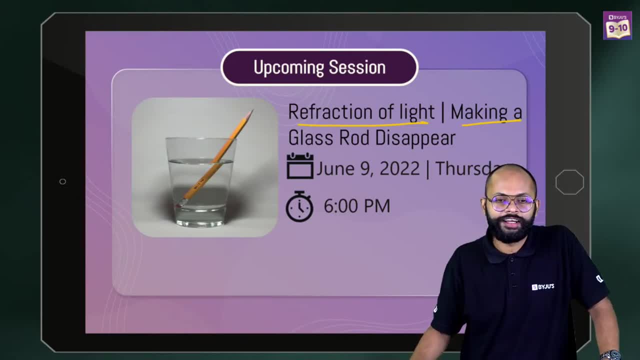 have taken the session again. new: every: you can use mirror formula straightaway. take V as infinite and take you as F. Yeah, Which you will get actually Right. Nice Arush, If we want to see it in the yeah, don't worry, I'll tell the team. It's okay. No, no need of two F, Yes. Next, 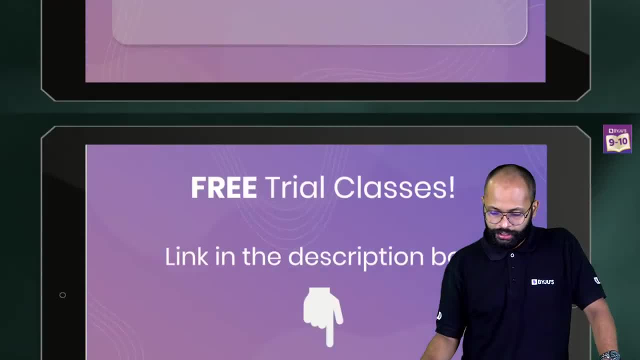 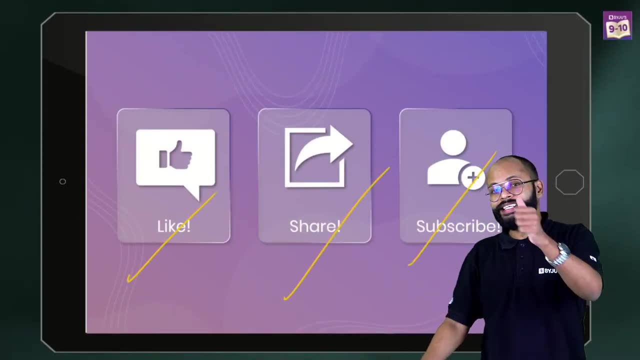 session is this, but yeah, we were supposed to do today, but next time we'll do it. A trial class is there, And you know what? This is the last thing which I tell you every time. I'm not saying just like share and subscribe That I'm expecting you will do.